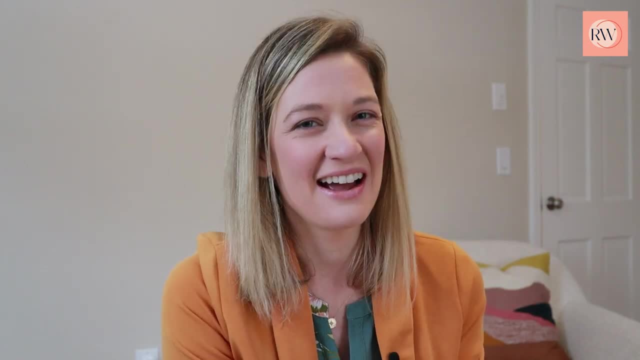 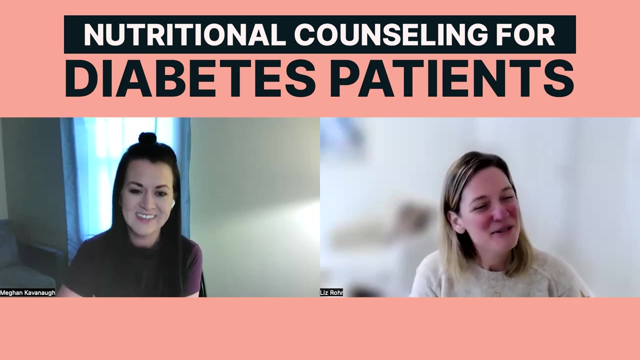 the best. So, without further ado, here's my interview with Megan Kavanagh. Awesome, Thank you so much for being here with us again. So can you introduce yourself to anybody who hasn't heard from you before? Yeah, sure, So I'm Megan Kavanagh. I live in North Louisiana. 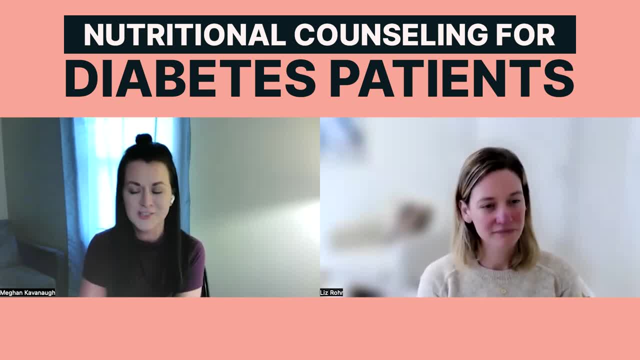 I'm a family nurse practitioner, but I'm also a registered dietitian, So I started my career as an RD and then eventually decided to go back to nursing school and then NP school. So I currently practice as a nurse practitioner, but I maintain all my credentials for RD. That's awesome, That's. 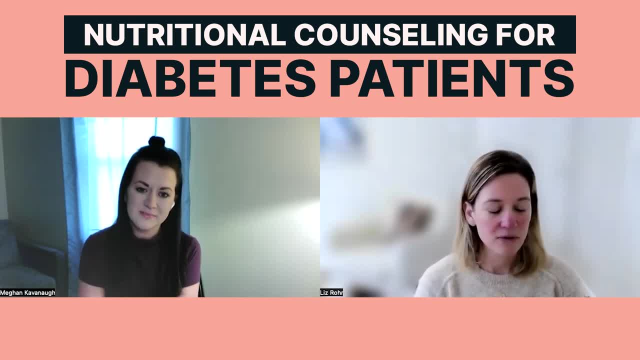 awesome, Yeah. so we did an interview- you and I did an interview for the channel before, for the channel as a podcast on YouTube- and we really focused on the diabetes care most common questions from a nurse practitioner perspective And so, even though you're not practicing as an RDN right now, 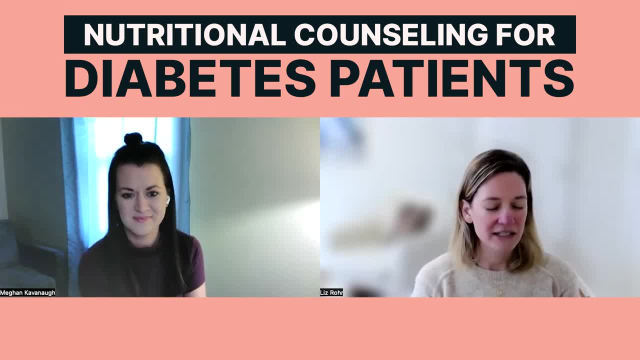 I'd love to kind of talk about, with so much that you have and so much passion that you have, Like, I think the context of the conversation- like you and I kind of just uh, just touched on before we started recording- was that so many? 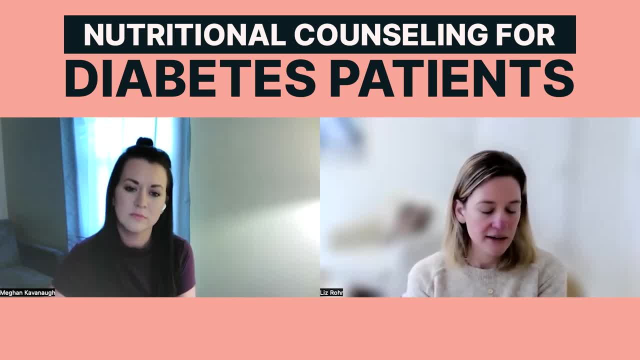 people. some people have a resource with a- uh, a nutritionist in their clinics. Some people have nothing, Um, and they don't even have somebody to refer to, And so a lot like what basically what we're, what we're going on are the questions from the real world, NP community And a lot of people. 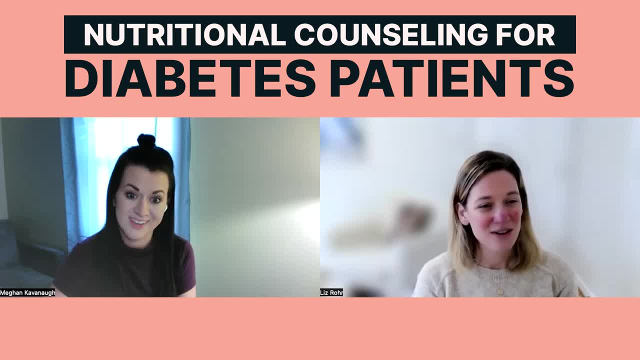 are asking questions like: oh my gosh, what do I do for patients who have diabetes and who need um support on the nutrition side? Cause it's a really holistic approach to diabetes. It's not just about medications, Right? So so thank you so much for joining us for this, So I think 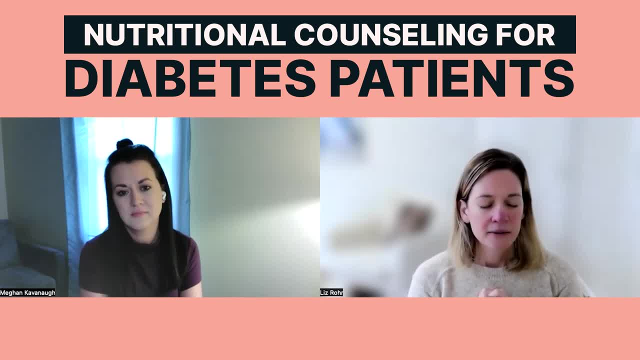 a place to start would be like what, as as in your, in your experience as a nutritionist- and you can obviously like add in your thoughts now being a nurse practitioner- like where? where do you start with somebody who has a new diagnosis? 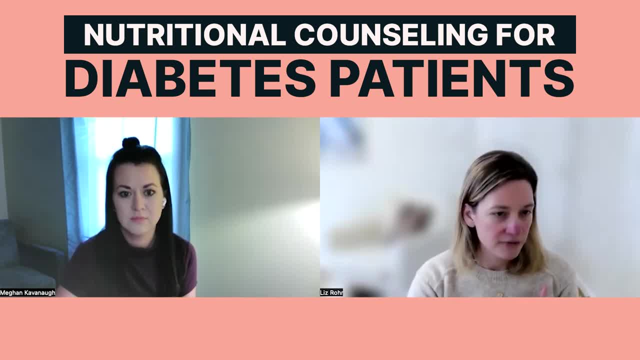 So, for example, if you're a nutritionist and you're a nutritionist and you're a nutritionist, for example, if I have somebody with a new diagnosis of diabetes and I refer them to your office and you were working as a, as a dietitian- um, where do you even start with a person in that? 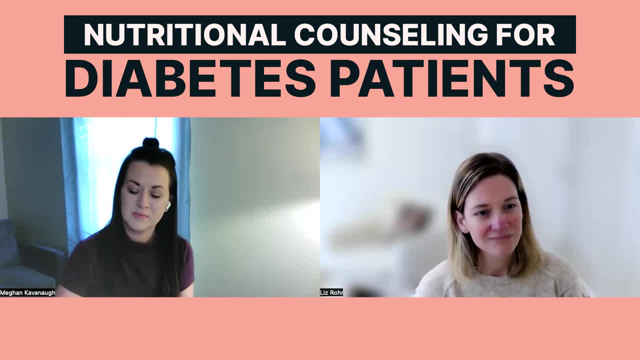 situation. That is a great question. It's a big question because probably one of the biggest questions the patient has is: what am I supposed to eat? What can I eat? You know what can I eat? That's like one of the number one things that's asked. 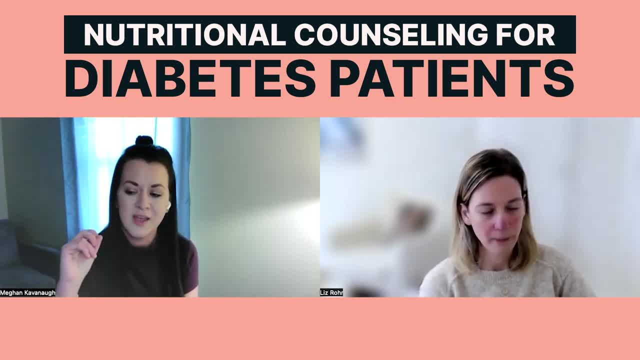 whether it be provider in um or RD or whatever, And the answer is like: you can eat a lot, You can eat all kinds of things And the where it's it's kind of hard to think of it now, you know. 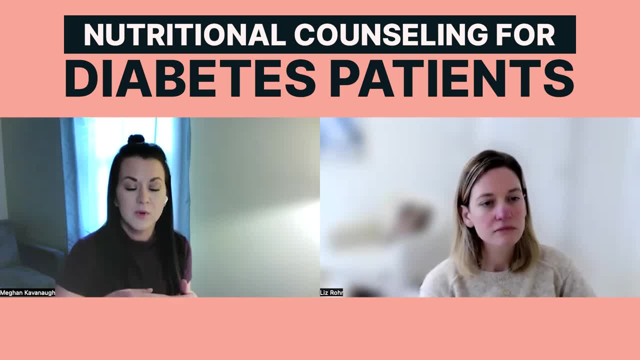 as an RD, because typically when you refer out one of the things, you have like a lot more time. Okay. So if you have as an NP, you're in clinic and you have somebody that's newly diagnosed and you are trying to start medications, start some initial education And then 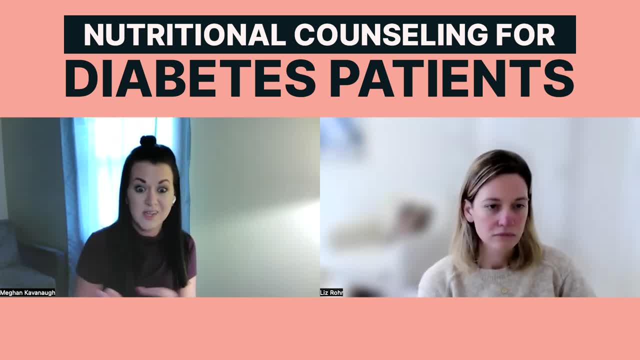 of course, nutrition is like on the focal point for a lot of people's brains. in what time of a time slot? what like 10, 15, 20 minutes, Like so? there's not a lot of time, So encouraging. 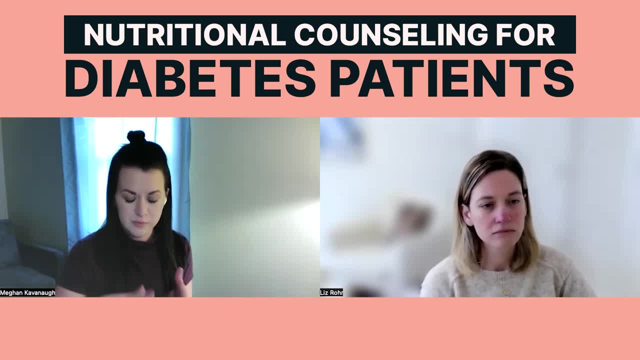 of course, to refer out, I really, when people especially say, well, what can I eat, I like to say: what do you like to eat? You know, I like started giving some ideas there And one of also from like the get-go, is just always reiterating that the you're not going to. 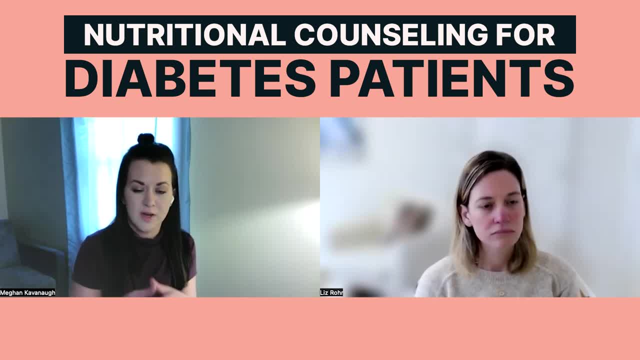 learn everything all at one time. Um, there's a lot that's going on with a new diagnosis with diabetes. There's a lot that goes on with nutrition along with it, And it's a huge learning curve. I mean, you might have somebody that's 60 years old and they've had 60 year old habits, And now that we're 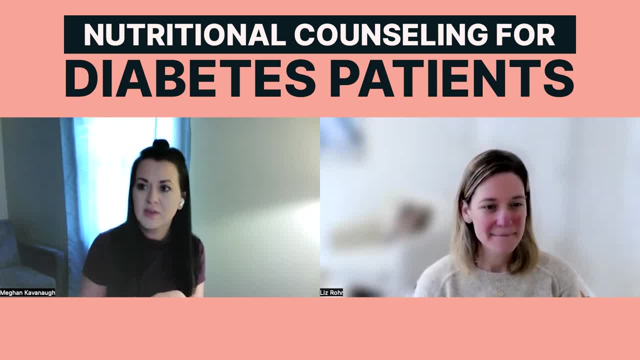 going to have to like transition. So it's a lot of motivational interviewing um, a lot of feedback, not just talking at the person but getting their feedback and building on that Um and then knowing, hopefully, if the resource is there, that they have multiple, multiple, multiple, multiple. 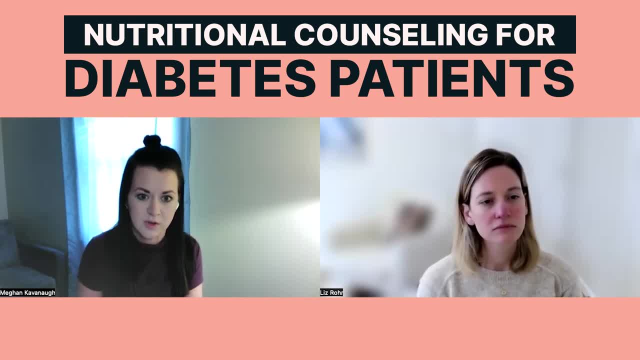 multiple visits to build on things and not having to change everything all at one time. So there's that's a broad question. I think that's a great place to start And I think it's so important to reiterate, especially for whether people are experienced clinicians, providers, um listening, or if 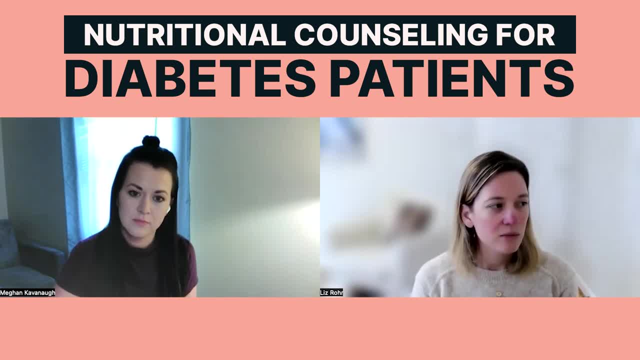 they're um. if students are going into practice like I don't know, that's my philosophy of practice too. Like you, and I share that of like. we just meet the patient where they're at And honestly, I think I feel like research supports that too, especially when it comes. 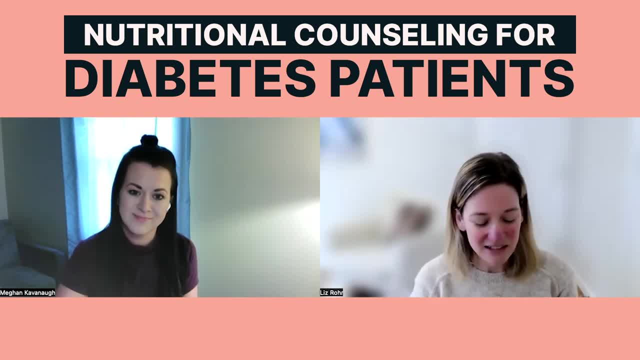 to motivational interviewing even if you don't feel super confident with that skillset, Like if you starting with where the patient is and doing an assessment first. I think applies to not only nutrition but also just like our approach as nurse practitioners in general: right Where it's. 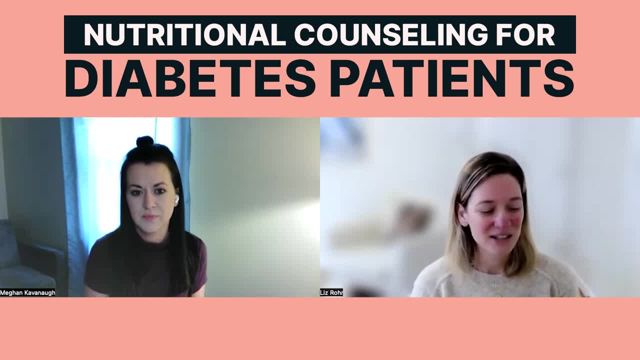 like: okay, well, where are we starting off from Right? Uh, so that's really cool. So I guess I guess the speaking from experience as a nurse practitioner working in a clinic- um, having worked in clinics where there's no resource in-house and we have to refer out and some people. 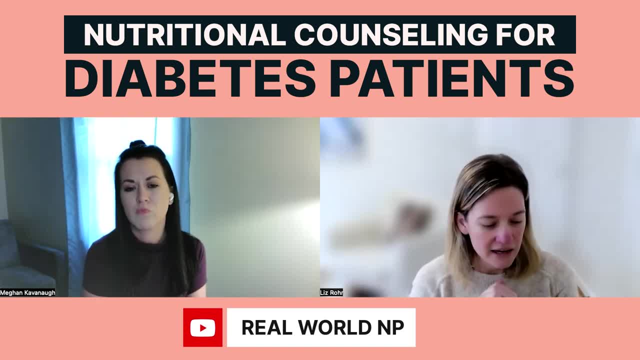 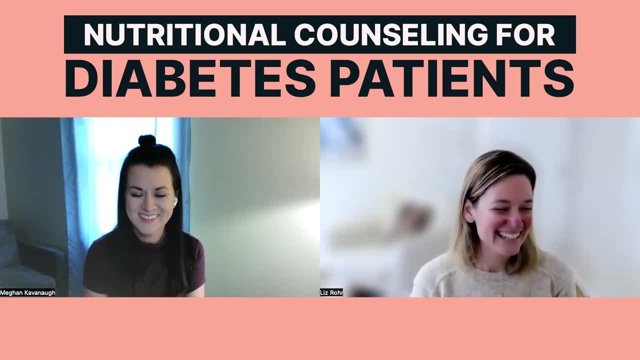 have access and some people don't. Um, I think that's a great place to start. And I think that's a great place to start, I think I think I can kind of sum up with the understanding that I have of the gist of what people do when they're in that situation. So I think that there's a couple. 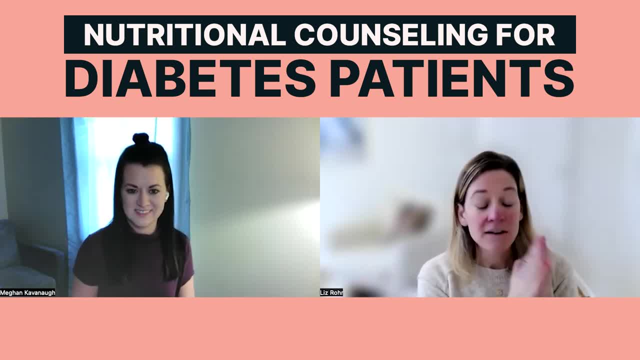 of things that people do, And one is kind of like, okay- And we also heard this from the questions from the community- It's like okay, so how, like where do we go? So if we've done an assessment with somebody, do we go straight to a recommendation? Cause, like clearly, you have a very 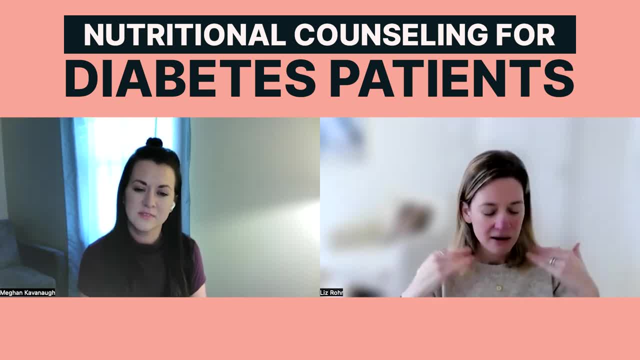 sophisticated nuance level of knowledge, Right, And so if we're talking about like moment, like starter place, one um is like, do I? a lot of people want to do, like, okay, do I do the plate method, Do I do the Mediterranean diet? Um, a lot of people wrote in and say I'm just, I'm tired. 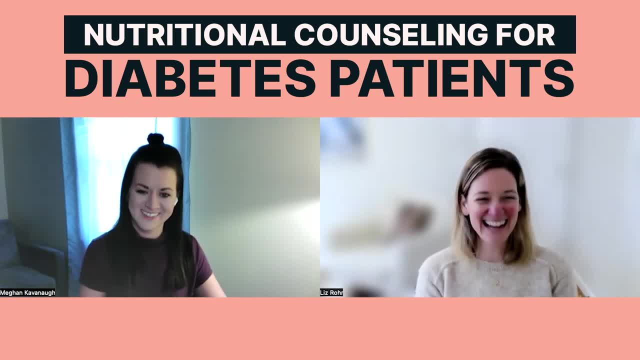 of saying: just eat less carbohydrates. Oh yeah, I love that part. Yeah, Yeah, And so it's like so. so, if so, where would you go in terms of like a first step, thinking about those potential three options of like? do you use the my plate method? Do you talk about carb? 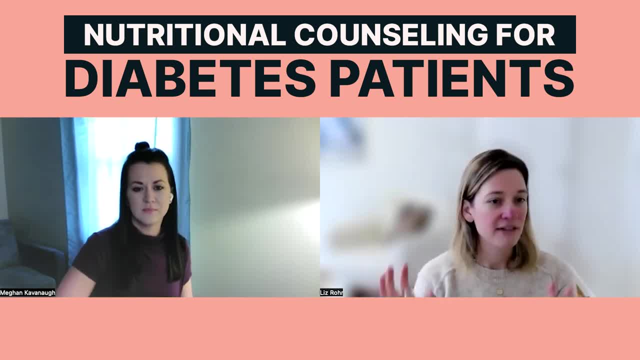 counting. Do you talk about less carbohydrates? quote, unquote, whatever that means, Like where what's like a first place to start, potentially for like a beginner one-on-one and a beginner one-on-one might start with? does the patient even know what a carbohydrate is? 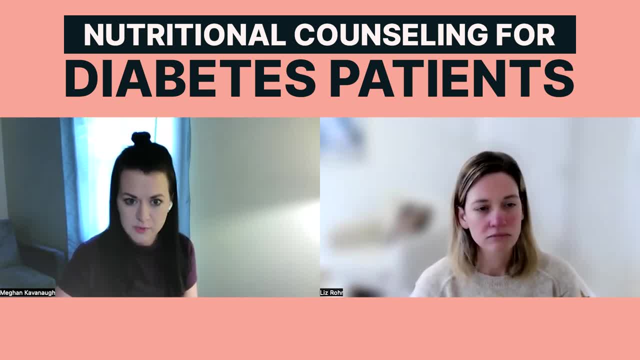 So they they might not realize that fruit can raise blood sugar, Certain vegetables can raise blood sugars. We- I mean we don't want to go in in any situation just like with that assumption that somebody has the baseline knowledge you know. So like tell me, tell me about foods that. 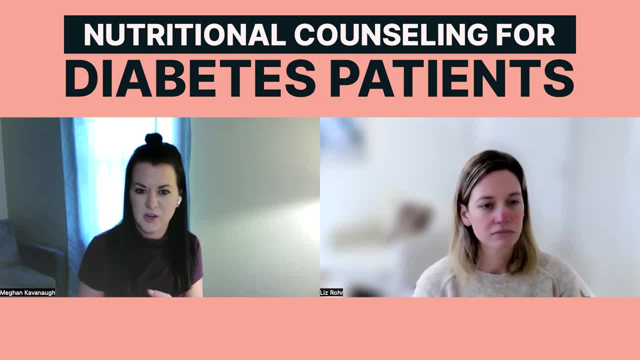 you like food, your um habits? Are you a snacker? Do you work night shift and you snack throughout the night to kind of stay awake? Um, do you have any different religious beliefs, cultural beliefs? you know just things. 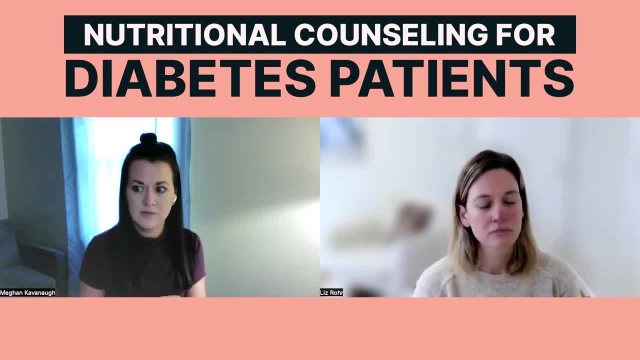 like that, Because everything that you read about nutrition is right That it's not one size fits all. So if you do say, okay, let's start with the plate method, Well, that's a good starter. It's a good visual for a lot of people, It's very easy and it's adaptable for, like, a lot of. 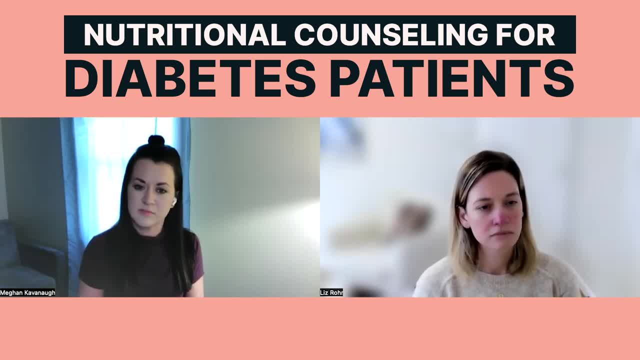 situations and meals, but like Mediterranean diet it's very, very healthy. That might work for some people Versus just explaining what carbohydrates are and like the focus at the beginning of like reduction in carbohydrates. So you do have to get a little bit more of a history at first to kind of 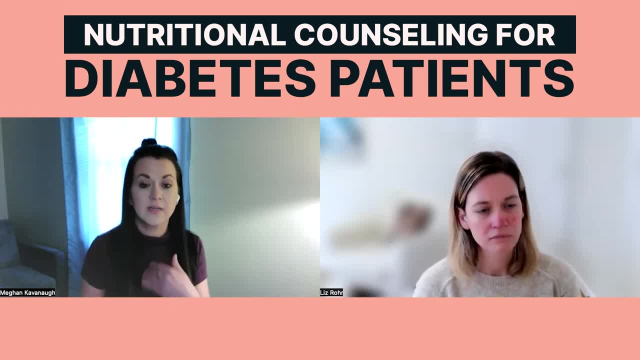 figure out where they're at, because if they're newly diagnosed- like for, for instance, for me, like if they see primary care, they're newly diagnosed and then they see us soon after that- Well, they've already probably been on Google and like looking at things, and you know, they might. 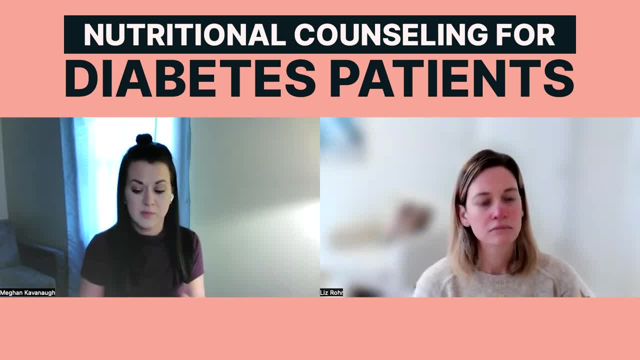 have a family member that is teaching them some things. So by the time they've seen us, sometimes really good changes have already been made. So you know, I think that's a good start. Maybe they're drinking a lot of sodas and sweet tea and juices and they cut that out and they've had 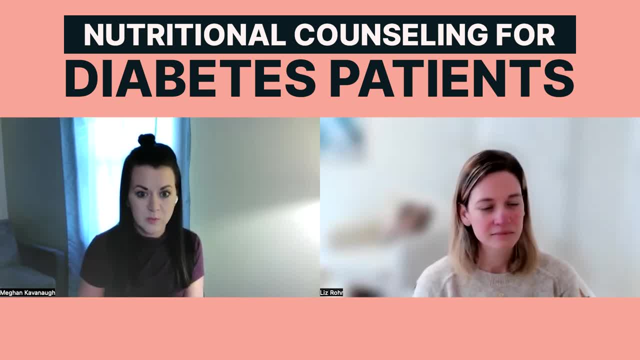 a significant improvement already. So again, it's just like meeting them where they're at, but it is when you're limited in that time it is very like: okay, I'm just going to do the plate method and just start with some education there, but it might need to start with okay. 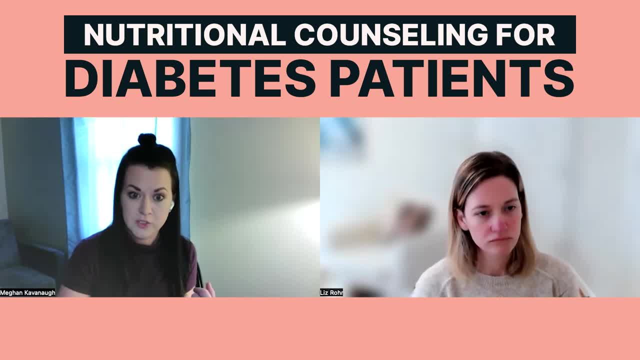 let's just focus at first. Are you drinking any sugary drinks? Okay, That's an- I say easy. It's difficult for people to do that, But if you're limited in that time it's very, very easy to do. but right out of the gate it's like: Hey look, even if you are still having some higher. 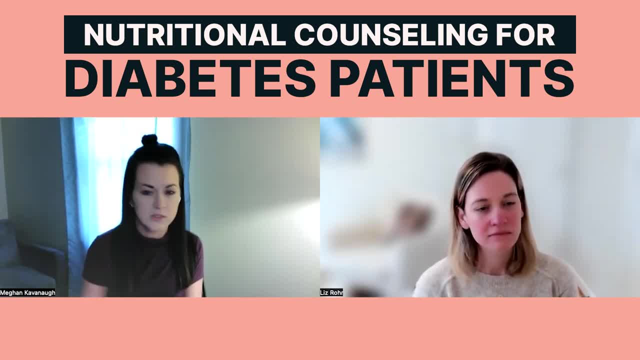 carb meals, but if you're having sodas with it or drinking tons of juice or even large quantities of milk, let's work on reducing that, because you're going to see an improvement pretty quickly. So that's a good starting point for a lot of people, And even if you have the ability to have 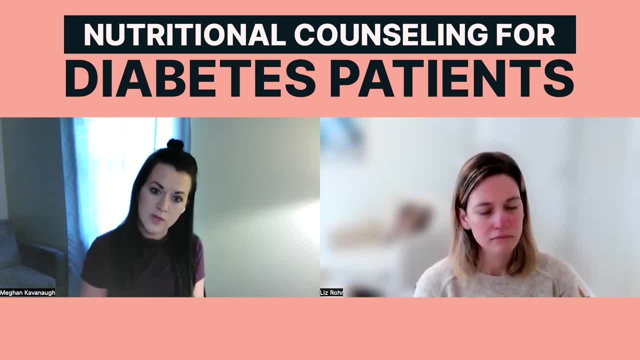 a regular follow-up with somebody they can keep track of, like even little food logs, or use something on their phone, their notes app or an app where they can log some things so you can look at it. But again, that's where ideally you would have a registered dietitian doing that. But of 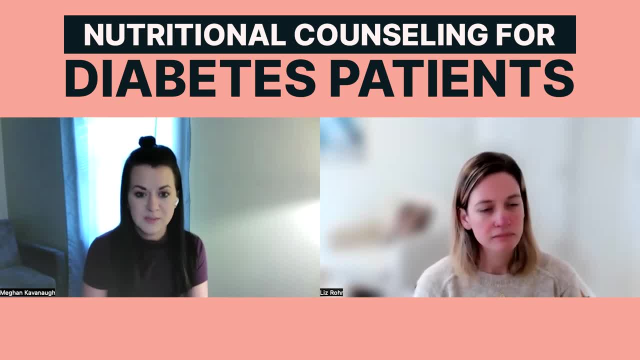 course, not everybody has that resource. So it really just- I hate to say it depends, but it really just kind of depends on where that person is. And then a lot of there's good resources online, like good starting places where, like, even if you say, okay, I'm going to get you in with an 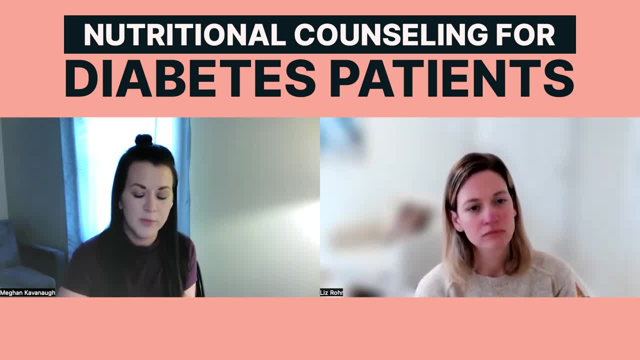 RD, but here's a good resource That can be printed off from. you know, American Diabetes Association, AADE, has a good one Diatribe, which I can give you. the links for those And, of course, like the MyPlate. 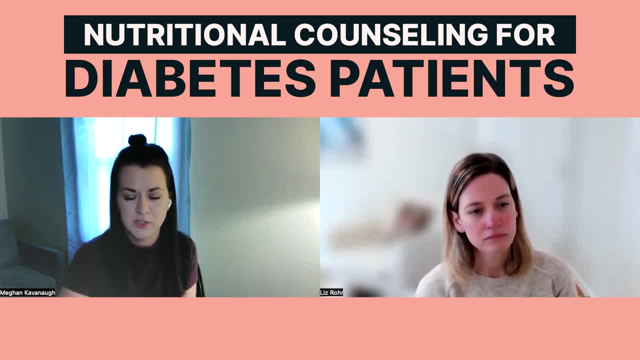 but something that's a good visual, that's basic, just to start getting some education for that patient Totally. Oh, I love that. Do you feel like? is this? my intuition is that it's also a patient dependent thing, but do you feel like, are there any sort of like standards that you? 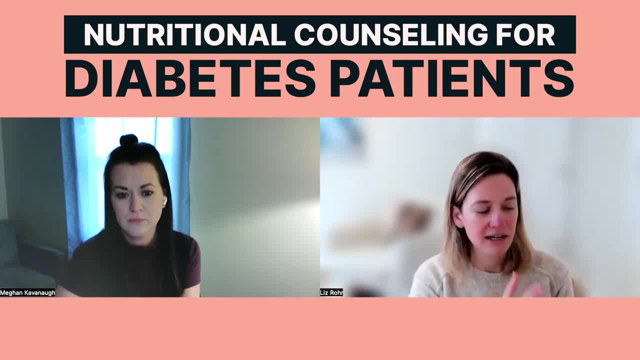 follow as a, as a dietitian, or the dietitians follow where it's like: oh, I'm going to get kind of like: here's the ideal amount of protein, ideal amount of carbs, ideal amount of. you know, like is it? is it? does it ever break down like that? Or when you come and you do a follow-up with 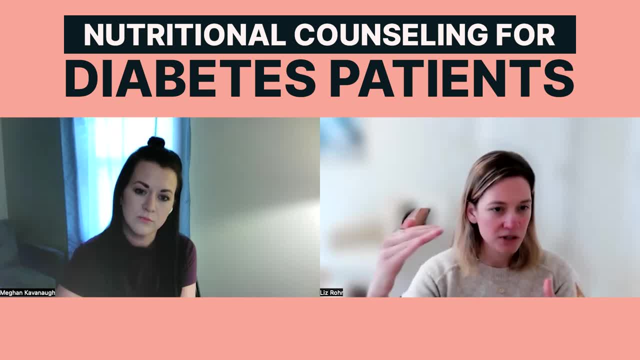 a patient and you've started at that place with them when you do their follow-up and their blood sugar maybe has improved but it's not getting. it's not like at goal yet. Like, where are your places to go for that Like? are you like what is leading your thought process there, Are you? 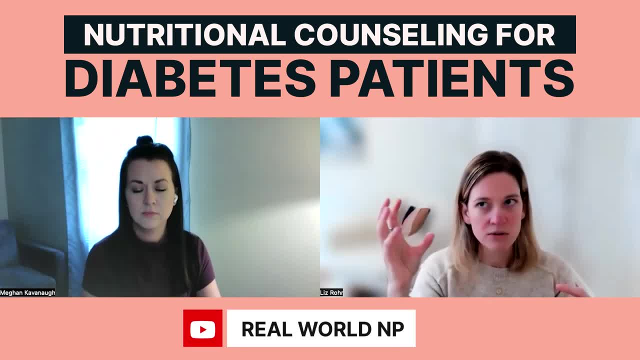 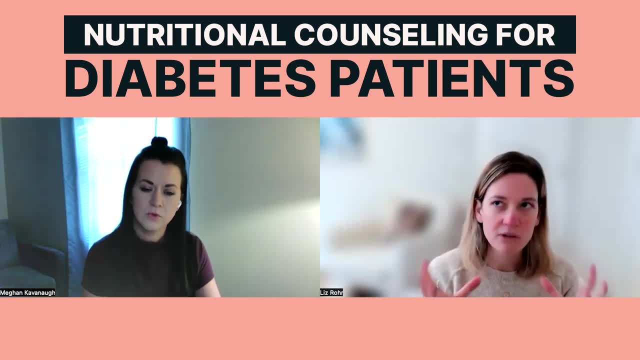 looking like it sounds like you're probably going to assess what their meals are, but are you just, are you simply targeting carbohydrates at that point? Or tell me a little bit about when it comes to the if you've started so, for example, if some if in the primary care clinic. 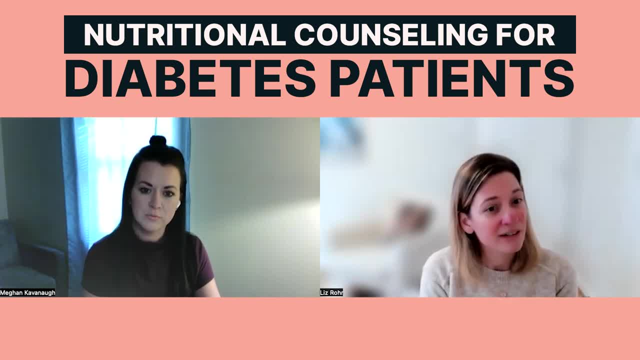 you start with reducing milk, which actually has a lot more sugar than I think a lot of people realize, and juice and sweet tea and stuff like that, And so does so say they've made that change and they're not at goal. Where's that next place that you're kind of going with that person. 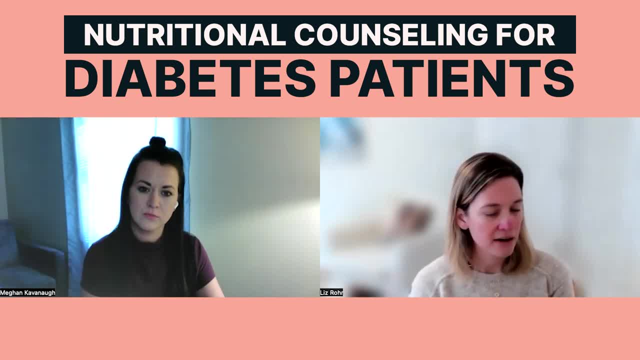 Is there an ideal or is it really targeted, based on that person and their specific A1C, For example? it's. there are different targets and it depends on the guidelines that you read for different percentages of calories that come from the different macronutrients- fat, protein. 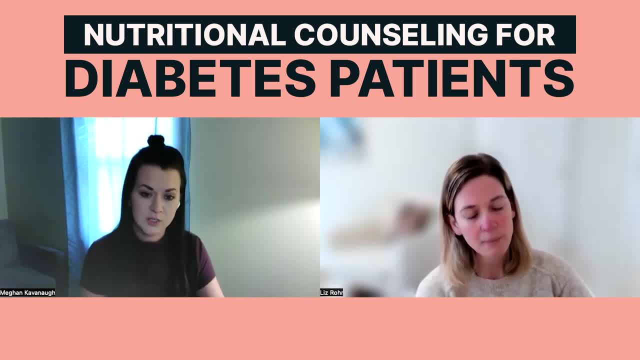 and carbohydrates Used to. I mean, like even when I was finishing RD school, like the amount of carbohydrates that were recommended were just like wow, Yes, it was a lot. And so finally, it was like I don't know, it might be a year or two ago- They finally said, Hey, a very low. 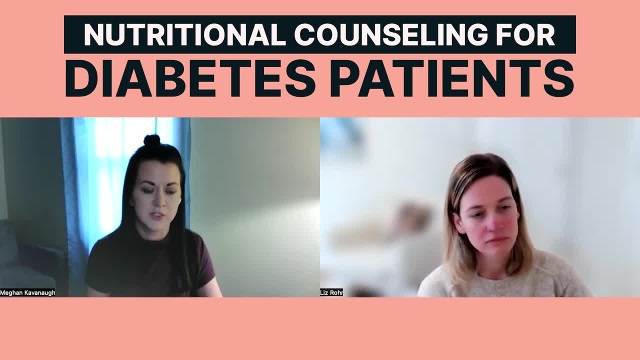 carbohydrate diet can be appropriate for certain patients and populations. And with your question, okay, Percentages for there. I also just assess with the patient how detailed they want to be, because when you start getting into like macro counting and if you're wanting them to count every gram, 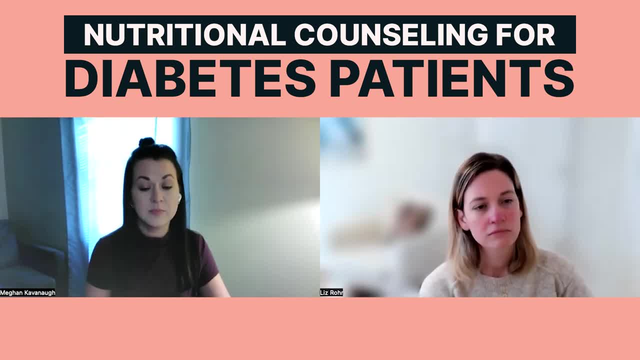 of everything. that's a. that's a. it's a big job and not everybody wants that amount of data And it's also very, very time consuming to teach. So but yeah, there are depends on the patient, their goals. 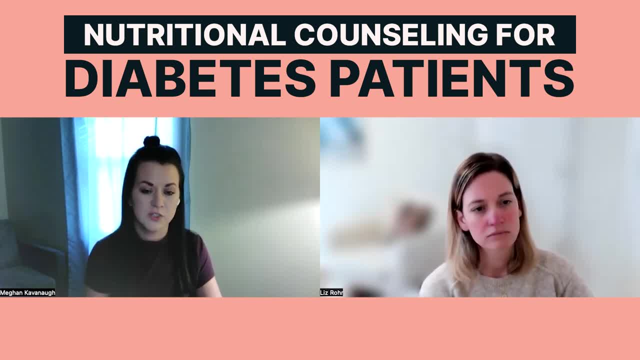 So you know, if they need weight reduction as well. percentages of each macronutrient, then kind of going from there and you can convert it into the number of recommended carbohydrates, like per meal, you know. so that's kind of a good starting point. 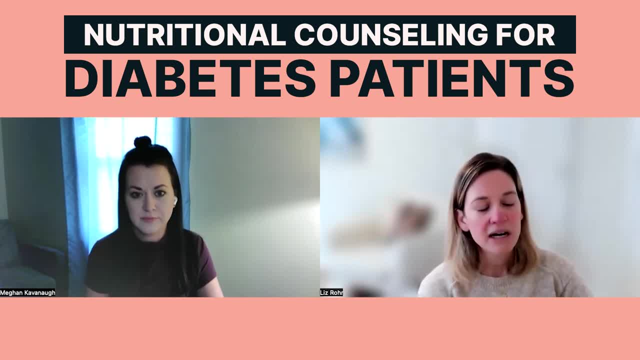 especially when you're getting into carbohydrate counting And carbohydrate counting My understanding is it's really most appropriate for patients who have type one diabetes. but what are like? tell me if I'm wrong there or what your general thoughts are from that dietician perspective about. 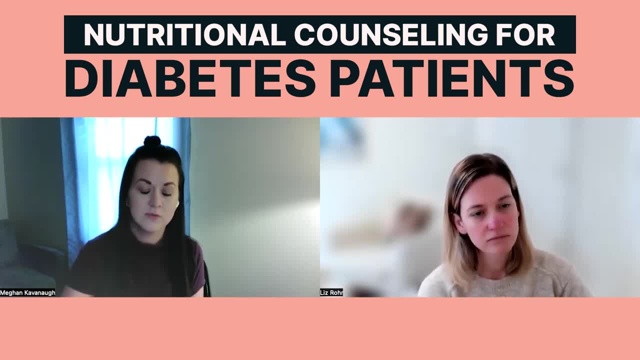 Yes, for type one for sure, because ideally the the carbohydrate counting, knowing how many grams are consumed at the meal, whether it be 12,, 26 or 64, it's converted ideally with the math for an insulin to carbohydrate ratio, So that patient is dosing their insulin based off the carbohydrates. 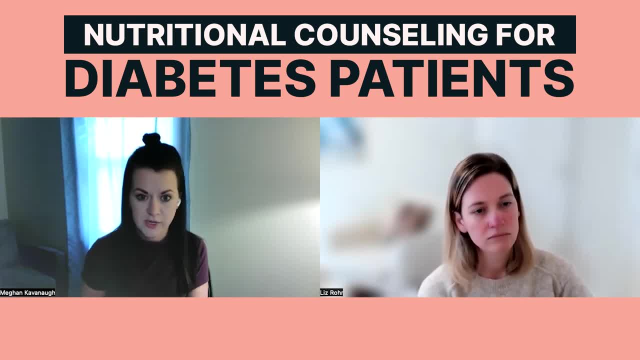 that are consumed. But we also do like carbohydrate counting for people who have pre diabetes, type two diabetes, because it's Mm-hmm, not even to be like so precise for that insulin dosing part of it, but also to be cognizant of. 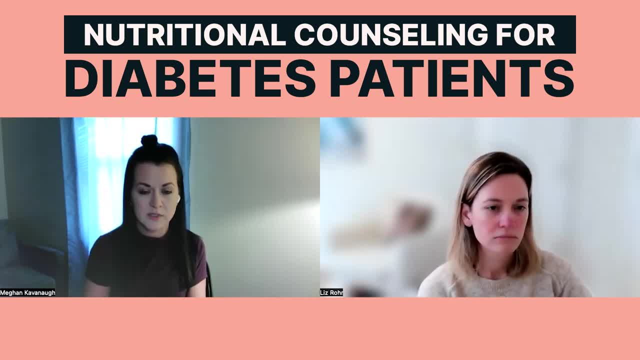 foods that can potentially raise the blood sugar and the amounts consumed it at that time. So we do with that, we'll teach that, but maybe not as to like a precise amount where if you have somebody that has type one or type two, that doses for an insulin to carbohydrate ratio and let's say 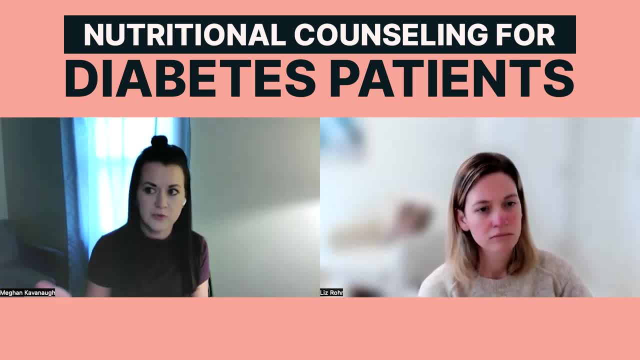 they're very insulin resistant and they need one unit, for example, for every four grams of carbohydrates, which is pretty strong, That's two saltine crackers. So you say, okay, well, if you eat two saltine crackers, that's one unit of insulin. So it's a bad precision. The 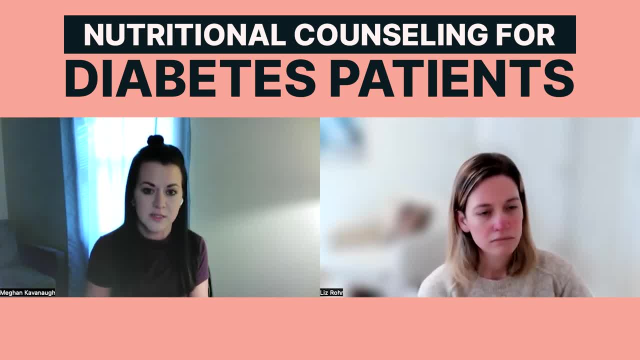 carbohydrate counting is very, very important and ideally done in the most accurate way possible for correct insulin dosing. Yeah Yeah, So that's pretty involved for most patients though. So I saw a number of questions and I've heard a number of questions, just like in in among mentees. 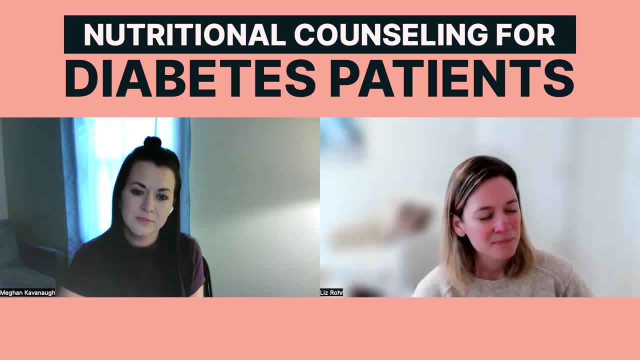 and in, you know, in regular life And stuff about what- different kinds of diets. So I think that there's different levels of health literacy depending on the patient, and some patients might come in and have done all this research and they might come in being like I'm going to do, like a ketogenic diet or I'm going 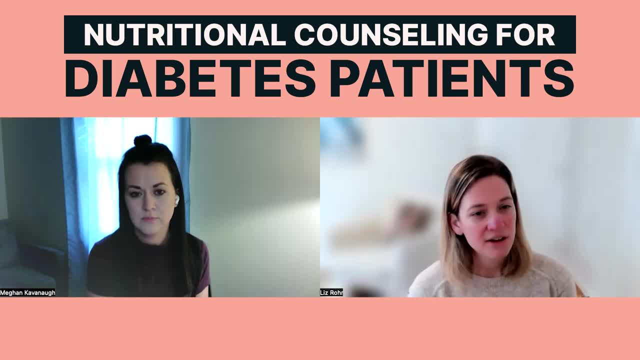 to do a paleo diet. I'm going to do a plant-based diet. Do you have any thoughts about that, When patients come in with that, with those kinds of approaches to their diabetes, or what kind of conversations with them when they bring that up with you? Right, And it's more? 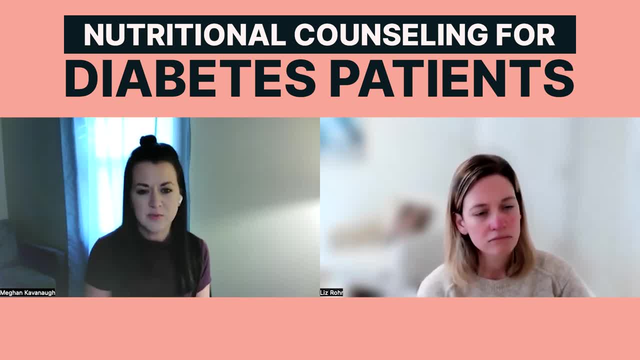 I think I think of it like more of an eating style maybe, instead of like diet, like kind of the labels on things or somebody saying, like you know, plant-based diet, but I'm going to be vegan, But every now and then I do want to have a little bit of animal-based protein. It's like let's just not. 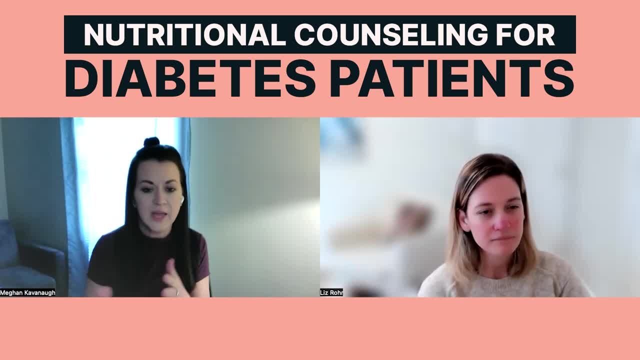 call it vegan, You know. if it's not more of a like an ethical type thing and you're just wanting to do more plant-based, you don't have to call yourself vegan Right, Or cause I like the term. like the flexitarian, you know just kind of different options. But 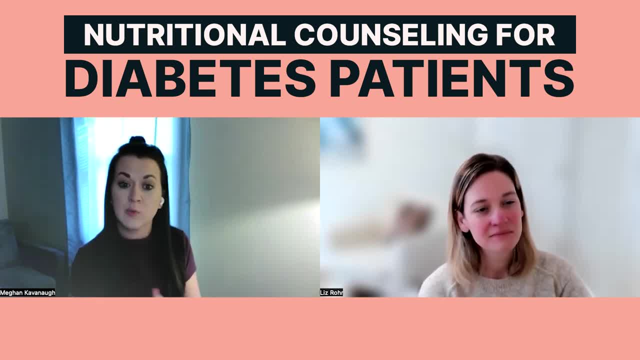 um, especially when you start getting into keto and somebody says, well, I want to go keto, and I'm thinking, okay, do you mean low carb? or do you mean like true ketosis, where you know it's a very, very high fat, very, very low- um sorry, carbohydrate diet? So sometimes people say: 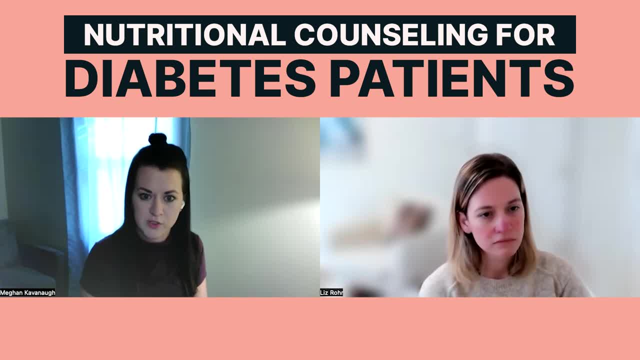 I want to do keto. They just really kind of mean I want to reduce my carbohydrates, Like I know I can, you know, lose weight doing that. So, and then I will also put back what they're typical eating behaviors are And it's like: do you feel like this is something that you can do? 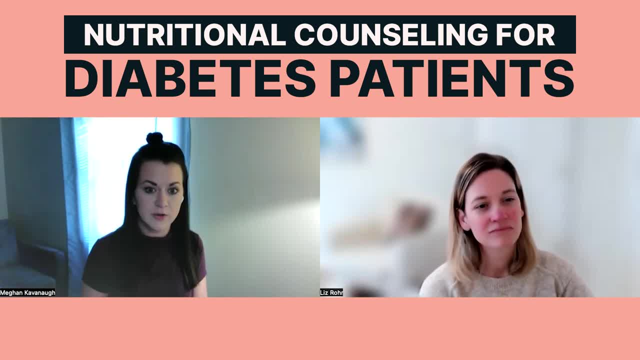 long-term. you know and we have you know. of course there's people out there that are highly motivated, that can stick with like a style of eating long-term. but I also want to reiterate to them that they're not failing if they don't eat that style seven days a week. you know every. 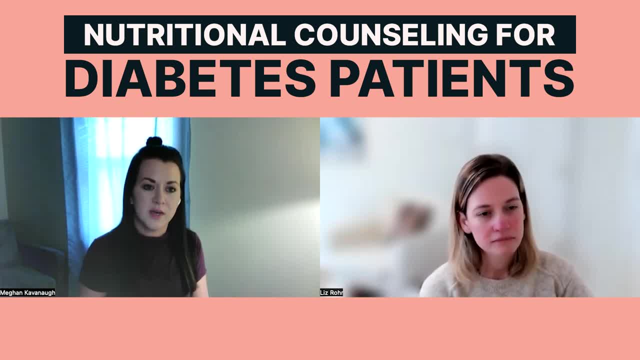 every week of the year. So with things like keto or low carb, low carbohydrate, I mean generally, especially if somebody is checking their blood sugars and um cause? we want to minimize hypoglycemia always, but if they have a continuous glucose. 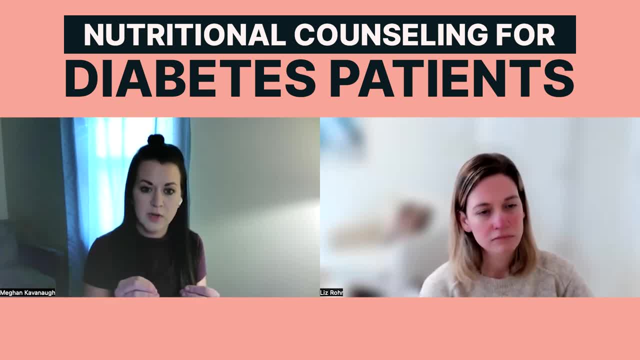 monitor and they're able to see the effect of carbohydrates, even low, moderate, high, on that CGM. a lot of them kind of naturally shift to like, wow, I had no idea that milk did that to me. or you know kind of the obvious stuff like cereals, like something that's high processed. 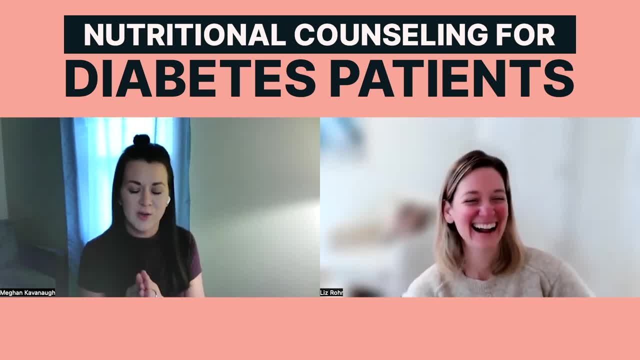 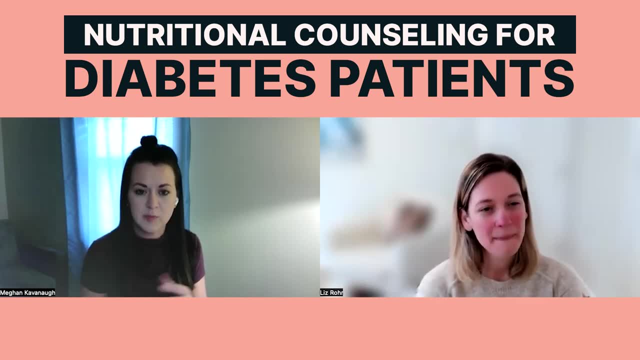 carb and you're like, Oh, please throw it away, Just get it out of the house. But, um, so they can look at that data and get more of like an instant feedback, whether it be through finger sticks or through a CGM, And it kind of you add some self-motivation that way too. Oh, I love that. 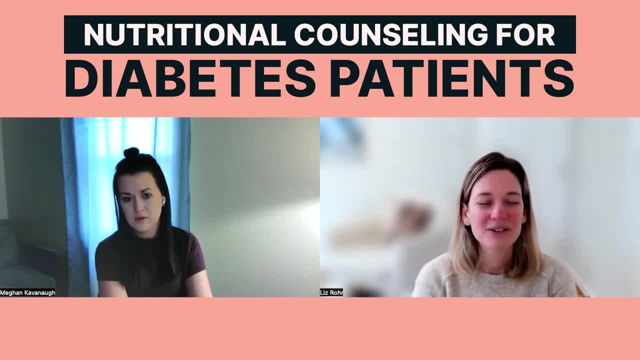 I love that. I almost wonder if you want to like, do a pretend patient, like if I was your pretend patient. I don't know if I'm staring my dietitian Like if I was going to be your dietitian. Yeah, Just like it's an example like how it would go. 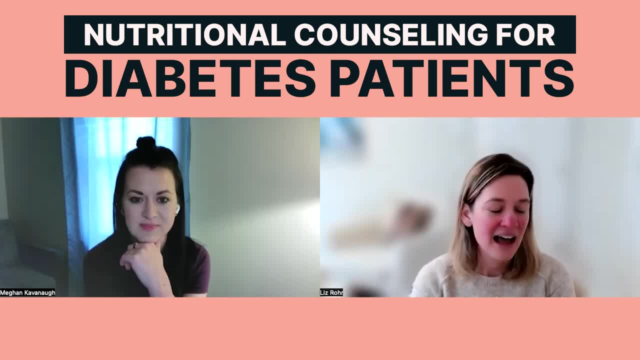 Yeah, Um, I guess, cause, like, I think part of it is also illustrating how complicated it is right, Because this came up with a physical therapist too, where it was like when I did a physical therapy interview. I think everyone's inclination, And I don't know if you feel this- 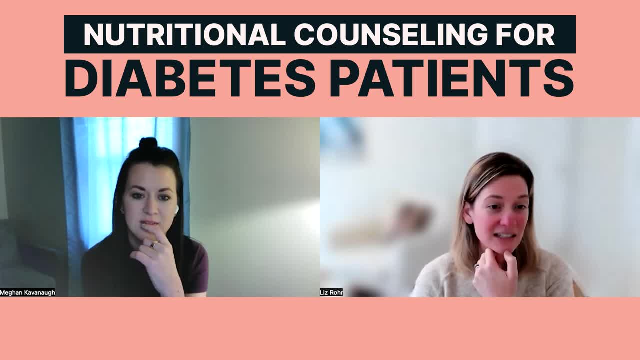 way too, is like: what exercise sheet can I give them to fix this problem? This is way more, way more complicated. Oh no, I mean, just like that question about the my plate versus. I just felt like I'm saying it depends for everything, but it does, I mean. 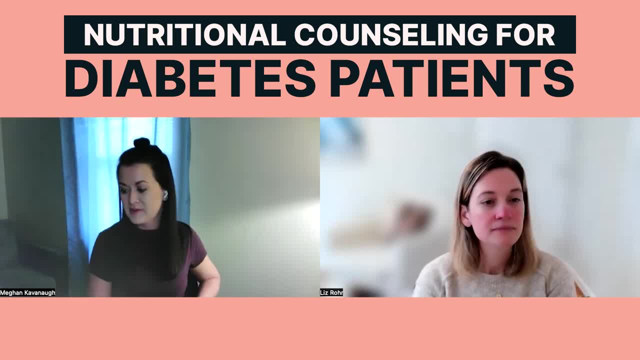 it does Like that's an honest, but people want to be like here's a sheet for this, Here's a sheet for this. Yeah, When I worked outpatient education and if it was somebody that came in just for weight management or type two diabetes management, um, I didn't have many patients at. 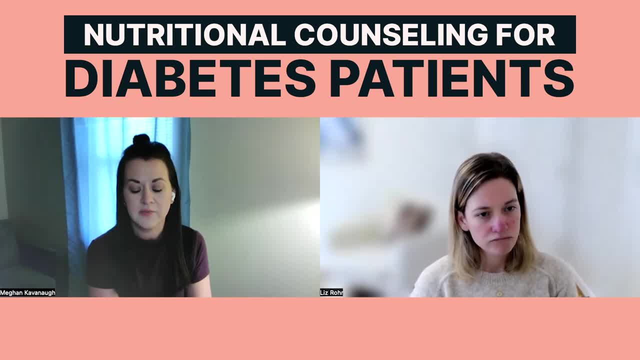 that time with type one diabetes. Um, they've. probably it was referral only, Okay, So when they came in they've already seen their primary care. We were education only, no management, and they would Um see the registered nurse either that visit or um like on the same day, or they would come. 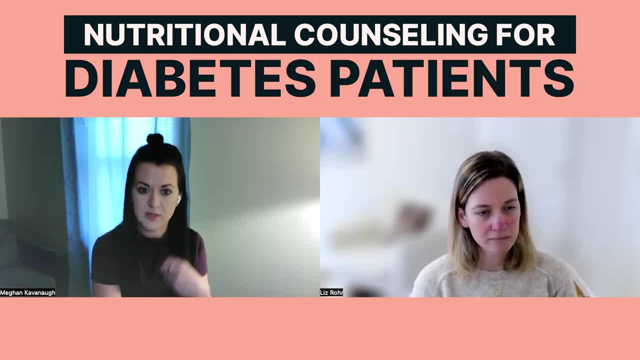 back another day with some food logs and everything. If somebody just like came in and they did not have any food logs, I started with: give me a history. Okay, What do you typically like? And I had these sheets and I said: okay, what do you typically like for breakfast? Give me some. 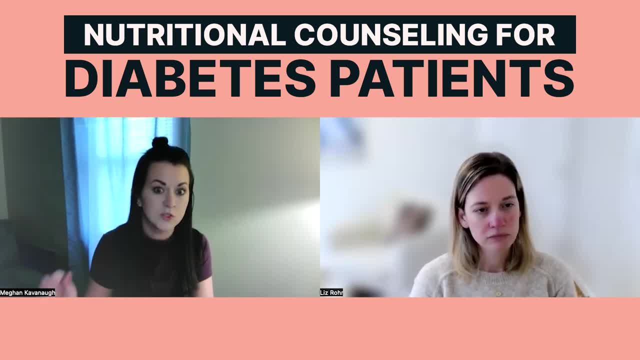 ideas. Do you eat breakfast? Jot it down, Okay. What do you eat for lunch? What's your work schedule Like? tell me about that. Do you snack? What do you snack on? What do you have supper Do? 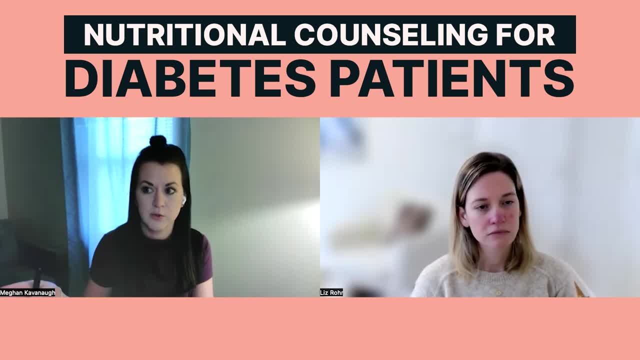 you skip meals? Do you feel low in between meals? Um? are you a stress eater, emotional eater? Are you a stress non-eater? And do you snack at night? Okay, Do you work nights? What do you do? How do you stay? 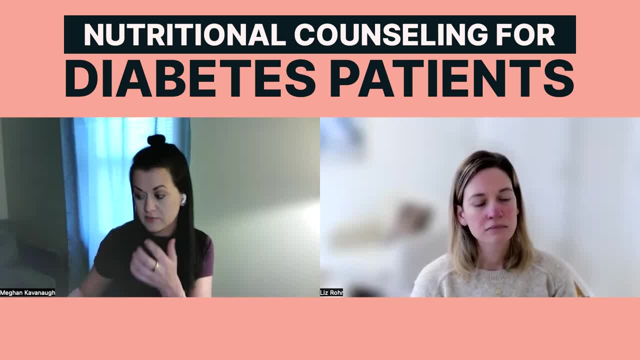 awake. What do you drink? How much? how much water, Like? you get this huge history, So I would have cause. I'm a. I'm a pen and paper person, Okay. So, even with all this technology, I'm just 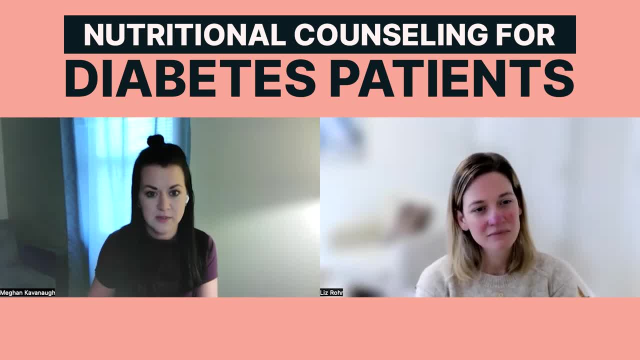 writing all this next time. So then I say, okay, look, this is your normal routine, Let's make improvements on this. Okay, So you drive a truck, you drive cross country and you have fast food and restaurants. What are your favorite fast food places? What do you like to get from there? Okay, You're not. 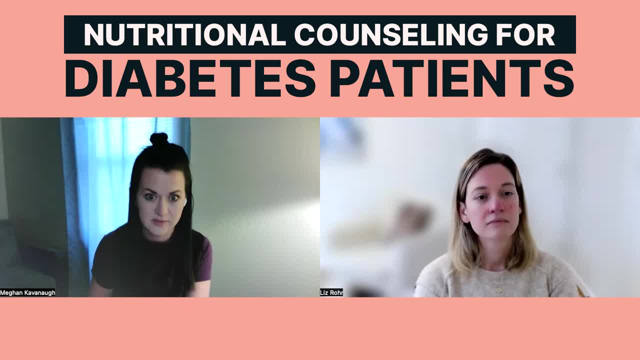 going to pack anything And then we need to do fast food, Here's what to get, I mean. so it was like examples based off of their history, Like at that time they came out holding something. It says, Oh, when I go get pizza, this is what I need to look out for When I go in. I'm working. 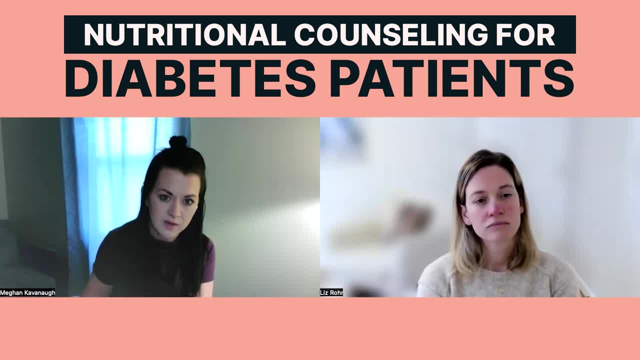 nights. These are some ideas of things that I can pack based off of the foods that I like. I mean so it's like very history based and then improvement based off of their current, you know, routines. So that's why it's hard to say, Hey, like my plate is great, It's a good. 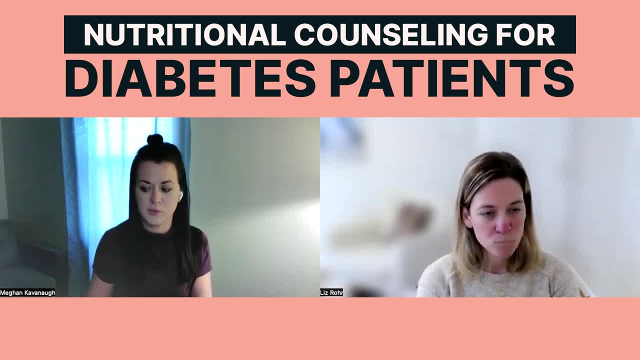 visual. but still, if you have somebody, okay, we do have plate vegetables, but the person's over here like I don't like any vegetables, What am I supposed to do? I'm not going to eat a single vegetable. What vegetables do you like? Well, I like green beans. Okay, Let's put some green. 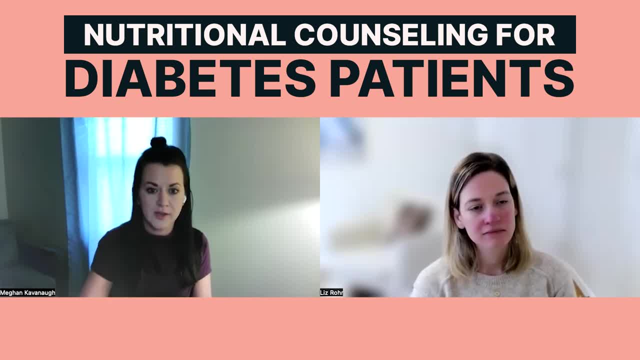 beans on that plate and let's build from there So you can be talking at that patient or like recommending Mediterranean diet and they can be allergic to fish. So it's like, you know, it's just um, it's more like history. That's why, like I don't even generally 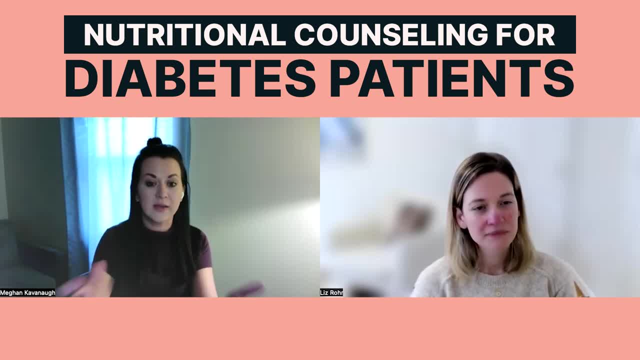 recommend saying like I don't say, Hey, let's do the Mediterranean plan. It's like, no, let's try to get good, healthy, fatty fish and let's get, you know, foods that reduce inflammation, instead of, like, calling it something. And that's why it's so hard, because, like, again, we want to hand. 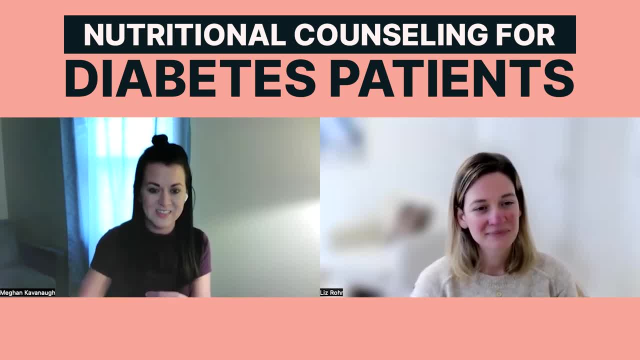 somebody, something that's just: Hey, eat this, this and this, which we have, the. we have the same handouts, but we've come up with them Like: these are the foods that will raise your blood sugars. These will help keep it steady, And that's still a good point, but it's like the. 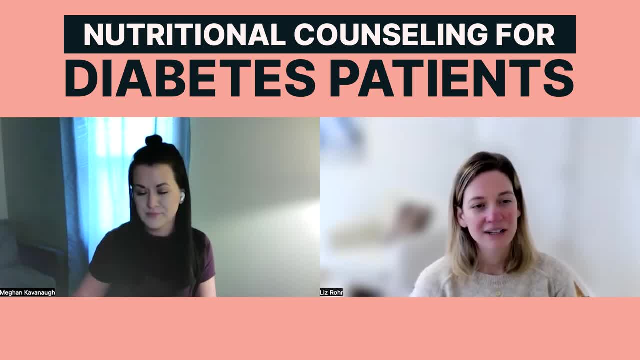 application to real life. You see what I'm saying, Like that's where I think that. yeah, I mean, I think that's the thing. like you know, with that physical therapy interview, everyone wants to give that handout: do this exercise when you have back pain, And it's like the hardest part. 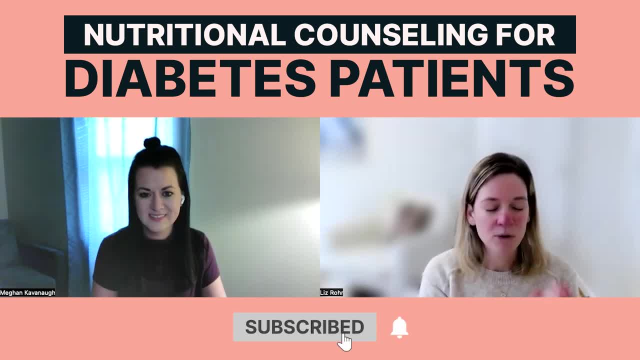 of like. I think for- and I'd love to hear your perspective on this- as both an RD and as a nurse practitioner For us, I feel like the the. the main challenge sometimes is the diagnosis or some conditions, And then, once you get there, the managements are pretty clear. right, There's. 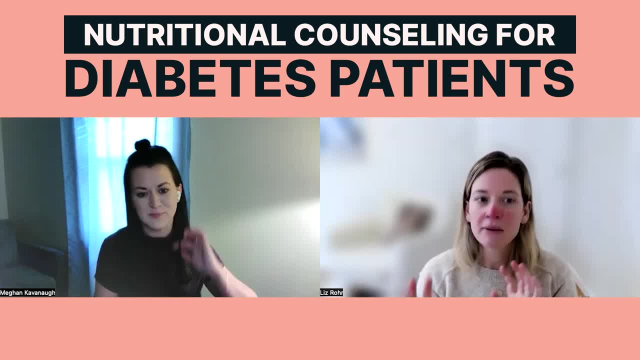 nuances and there's choices, especially when it comes to diabetes. right, Like you have to be a little bit more sophisticated nuance there, but for the most part, like I think that the main challenge at least newer grads and newer grad nurse practitioners have is like getting to the 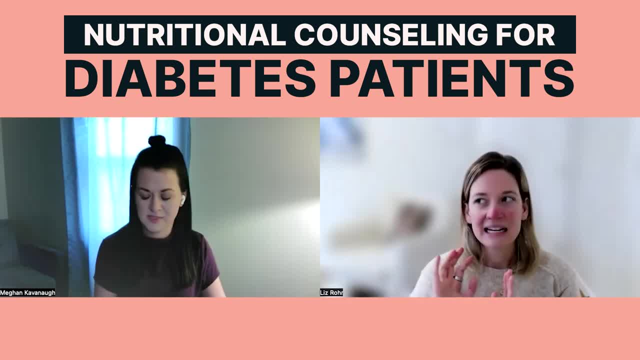 diagnosis and it's like, okay, what's the algorithm of management, Right? And I think that with RD, like I know for a fact from like doing all of that stuff and then doing that interview right- Is like, oh, that's the easy part, right? Is it an orthopedic problem or is it not? And if 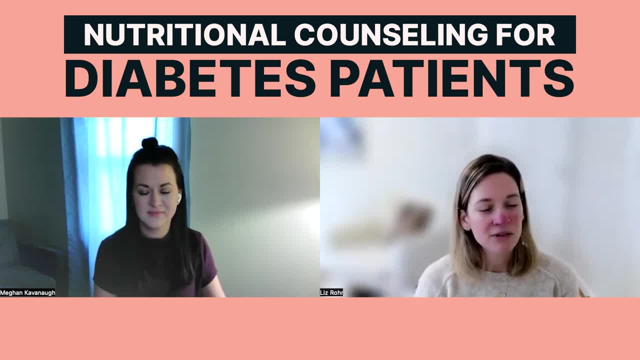 it's an orthopedic problem. here's all of the sophisticated management. So yeah, it really sounds like with RD, like that's, that's the same thing. but I love those history questions, Like I really love how much that illustrates why it is so um, why it is so sophisticated, And I think 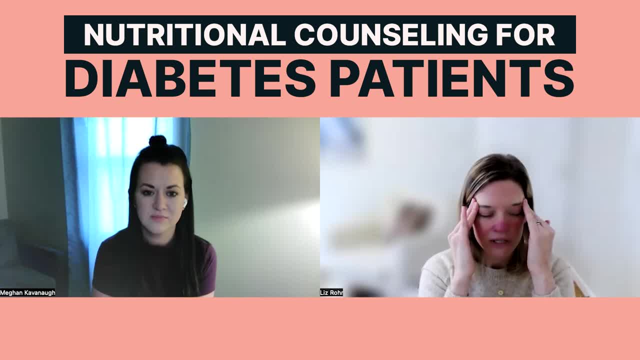 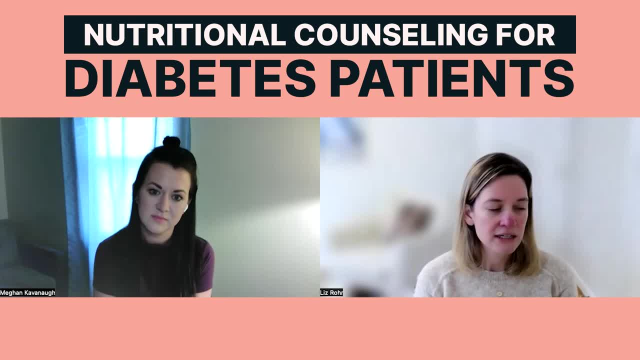 this from other people is like this responsibility to like take really good care of our patients in a system that is not set up to support patients optimal wellness. And so it's like, okay, how can I be an RD, How can I be a physical therapist, How can I be the specialist? Right And the reality. 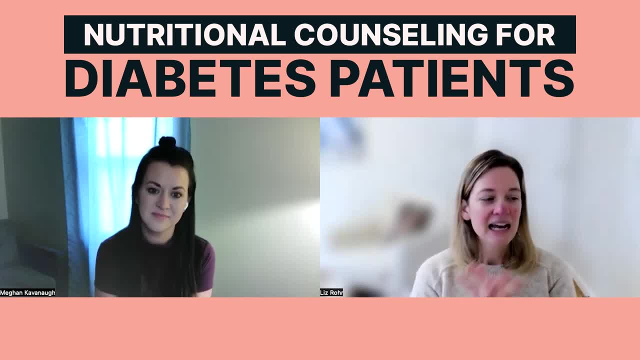 is we have to draw the line somewhere And it really sounds like with RD and dietary education, like there are places we can go And I think we can get better at of like what history questions to take. Right Cause, like I'm not asking things, like are you an emotional eater? Right Cause I'm not really like prepared. 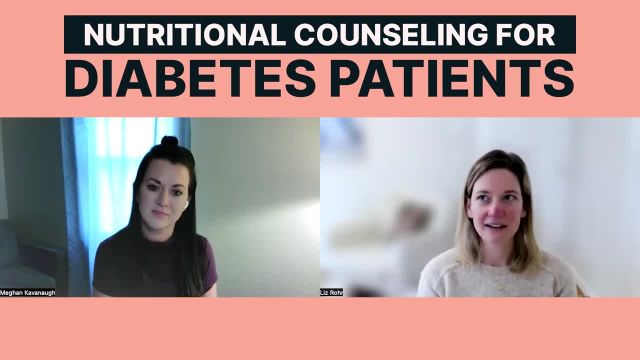 Excuse me to have that conversation of like where do I go from there? They answer, Yes, I'm like, okay, what do I do next? Right? And so it's like so, yeah, So I just I really appreciate that It. 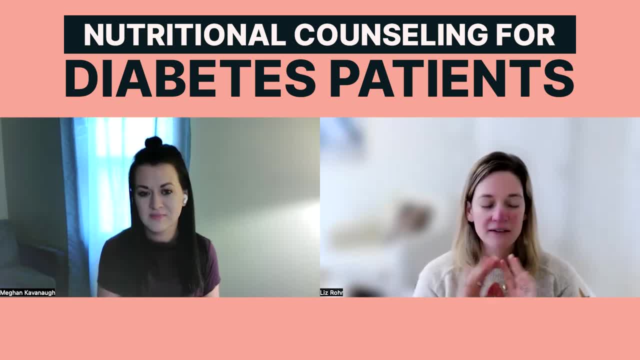 sounds like some places to go, though. um, with the knowledge base that we have as nurse practitioners is perhaps getting really comfortable. What are the blood sugar raising medication? blood sugar raising, Yes, Versus blood sugar lowering foods- Right. And then, how can we get better at the history and how can we develop our knowledge to be more? 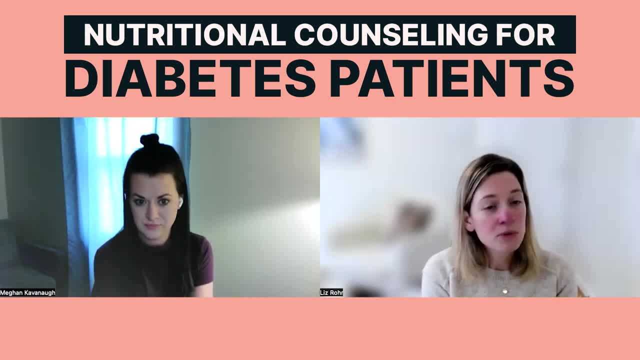 sophisticated such that we can take the fast, like. that's a beautiful, beautiful example- because that's real life right- Of patients who they're a truck driver across the country and they only get fast food. Like what other options are there when you're out, like driving, Like? 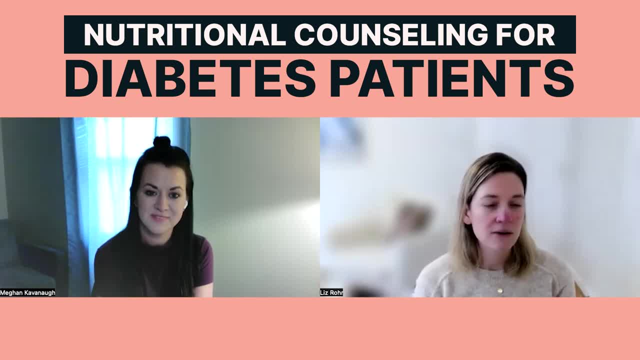 I don't know. I mean, I've been up on on really long trips where there's a lot of truckers and it's like, okay, well, here's one option in the next 45 miles. So, um, so that's. 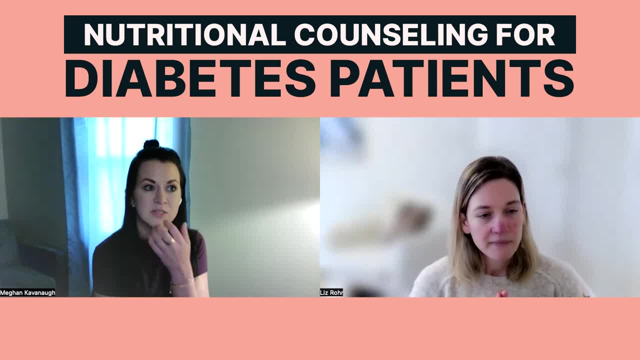 really that's really cool, that's really really helpful, and that is I mean you talk about like getting to the diagnosis and like where's the algorithm? I mean, if you and I compared like schedules, routines, um, you know, food likes dislikes, you're gonna get two completely different. 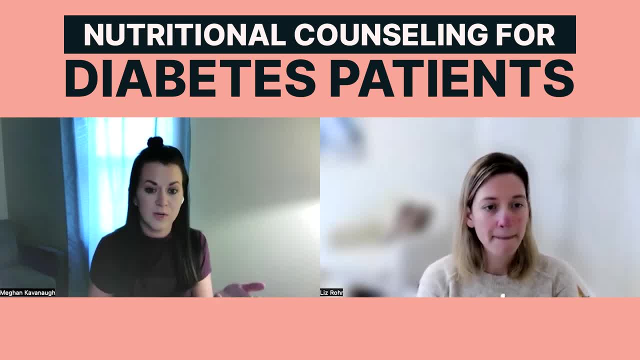 people on paper, right? so you know, right now my husband's traveling for work and I'm just making like an egg sandwich at night for supper because I'm not gonna cook a big meal and right now, just like in the season of life. yes, I know vegetables are very, very healthy, but they're also expensive. 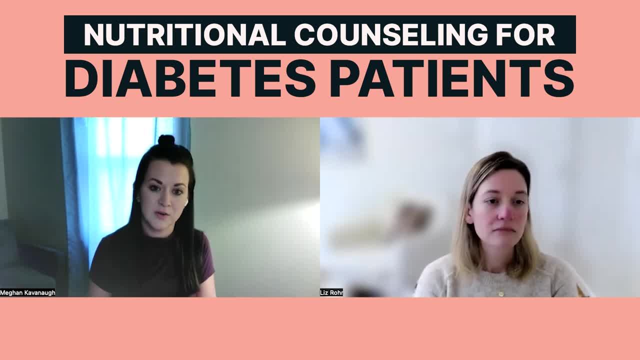 and they go bad, and you know so. right now I'm focusing on steamed bag vegetables that cost a dollar and I throw them in the microwave. they're done in four minutes. a little bit of salt and pepper, you know it's fiber, you know so. where you look at like even like social media, and like these, 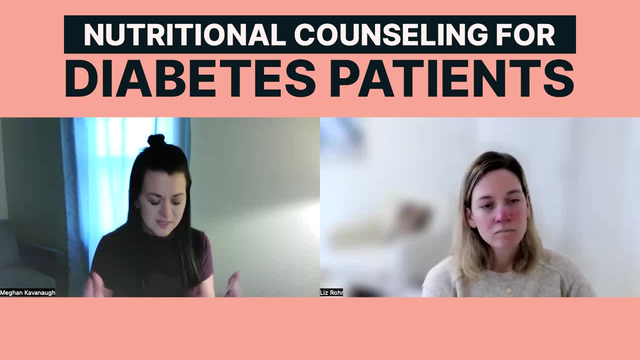 beautiful, like great meals. the always like telling that patient it doesn't have to be that complicated, it doesn't have to be that expensive food- I mean cost of everything obviously are crazy, but it's, it can be. make it like as simple as you want, while as nutritious as you can and doing the best you. 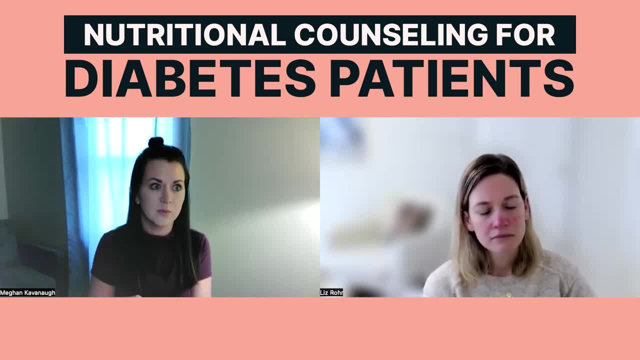 can in the season of life right now. I mean, it's like that's the takeaway. so we know every year holiday season, people are gonna indulge and have this like: okay, you know, if you have your grandma's favorite, like toète, the grandma makes the your favorite chocolate pie, okay, but you don't really care about. 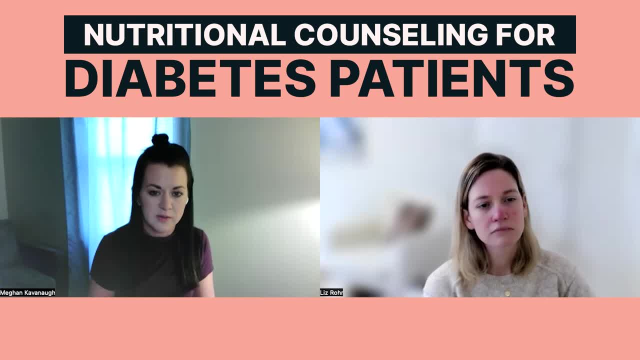 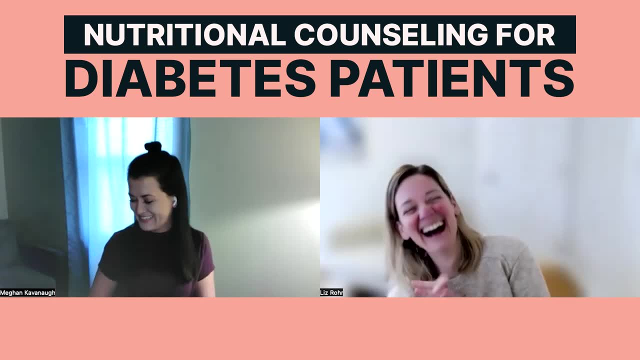 pumpkin. don't eat the pumpkin pie. eat the one that you like, maybe cut your carbs back a little bit, kind of acknowledge it. but make a holiday, not a hollow month. you know, just celebrate the day, but make it a whole month and you can still see improvement. so even these, a lot of these. 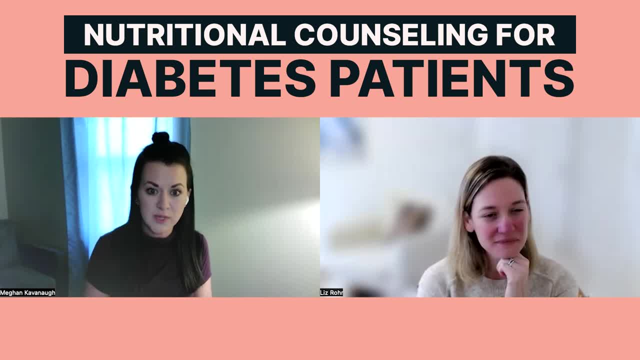 patients that come in after the holidays- and still have a lot of people that do- are having really good, consistent weight loss. they still have decent blood sugar control. there's some periods of time that get a little wonky, but it's like learning those little mechanisms of. 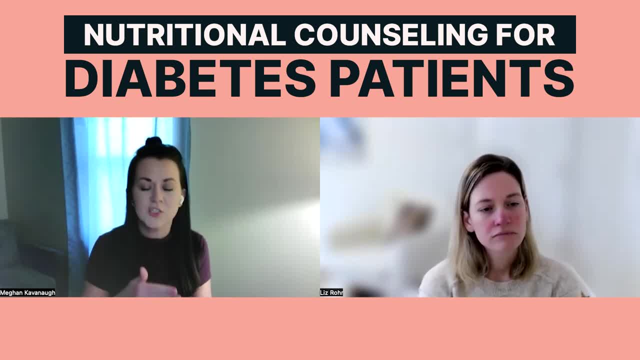 what do I do in the situation? what's the best decision I can make right now in the situation, the social environment that I'm in right now? and it might be a reduction in portions, like, if you can't control the quality of the food, control the quantity of the food, like just reduce it a little. 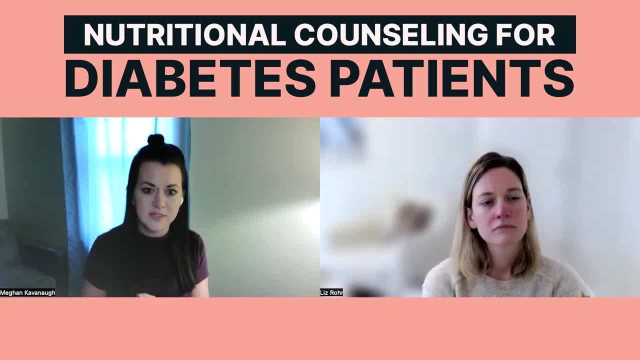 bit drink water, try not to overindulge in alcohol, limit it to maybe one sweet instead of three, like little things like that. you know, just over and over perfection, not perfection, but just improvement. you just want improvement and then, where they can see some success and kind of build on that and 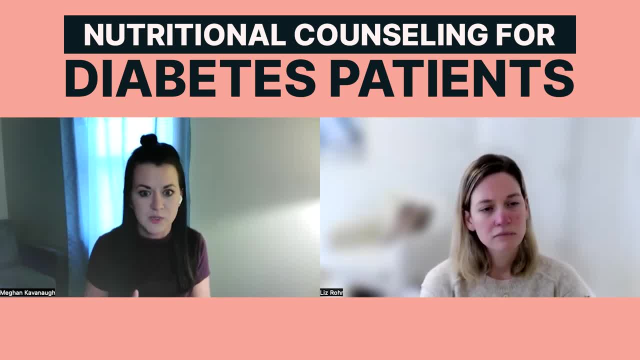 those are the ones that can really long term, have success, because they're realizing that I don't have to do exact macro counting to get everything right with the meds that I'm on in my routines and other things that we're dealing with. so I love that's. why, yeah, no, I love it's. 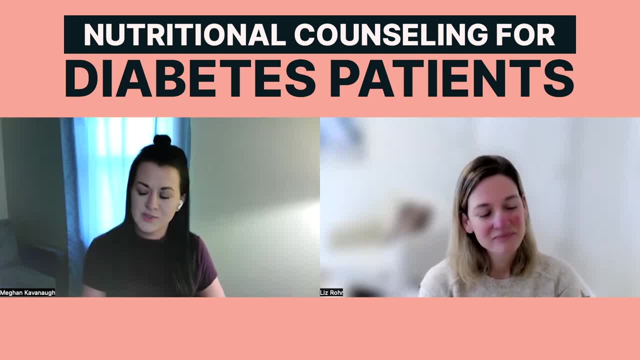 complicated and I think this is why you know, when I went back to nursing school and, um, some friends said, oh my gosh, our nutrition class is that I hate nutrition. I hate nutrition. it's really, it's hard and it's a lot of- yeah, hand-holding and you know it's food is very emotional. it's very easy. yeah, I mean there's 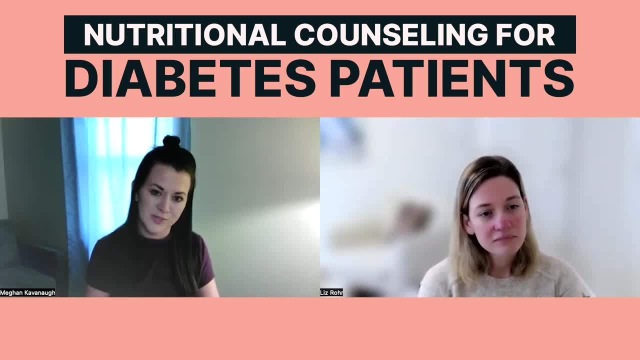 more to say you don't ask the question of like, are you an emotional eater? because what do you do with the answer: yeah, it's just like you need. it's like that whole like depression screening thing is like. it's not recommended to do depression screening unless you have the resources right and 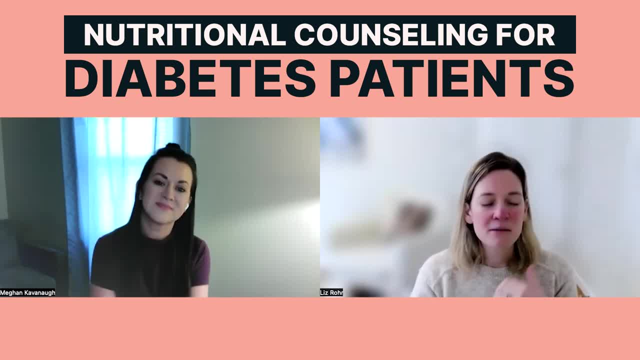 so unless I'm like in like, I can think through that and think about how I respond to it, but just like hearing you say that in the moment I'm like, oh gosh, like I don't even know- I don't think I've asked that of somebody before- and like, because I think like, especially like that's. I don't know if. 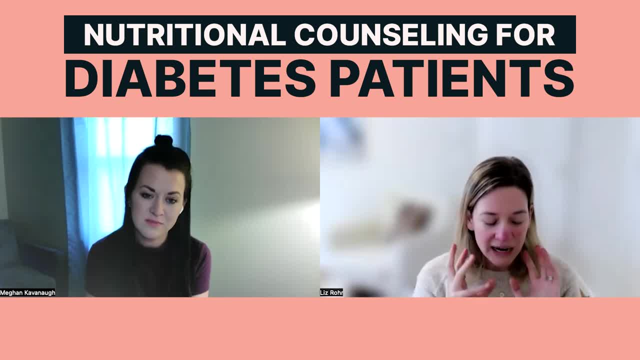 this is your experience. but my experience of becoming a nurse practitioner- like when I was brand new- I was really focused on like what is the safest thing that I can do, so I don't miss anything. and then, as I develop in my practice, I get into those deeper levels of sophistication. 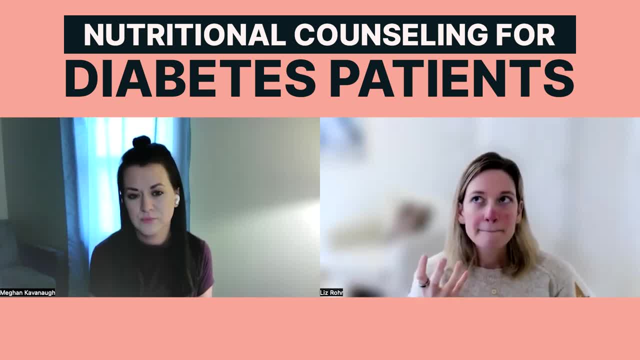 where one of the things I was going to say in terms of like part of it, like I think hopefully this is awareness raising and that, like one individual person- me myself, as a nurse practitioner- cannot fix a system that is not supporting the anti-wellness of our patients. basically, right and so, but like what are the things that I can do? 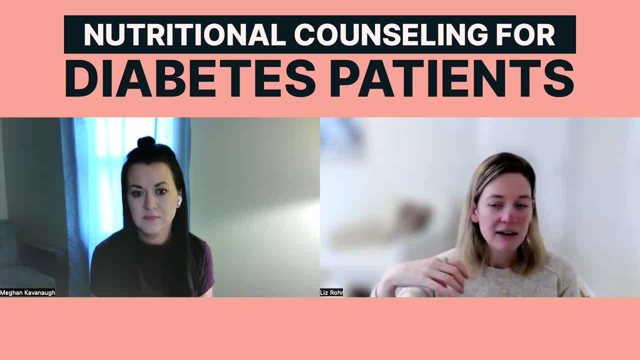 in my scope and how can I raise this as an issue and and talk about it with other people? like we need RDs, we need physical therapists, we need interdisciplinary collaboration for a reason, right, but like that's one of the things I was thinking about is like, how can, how can we like 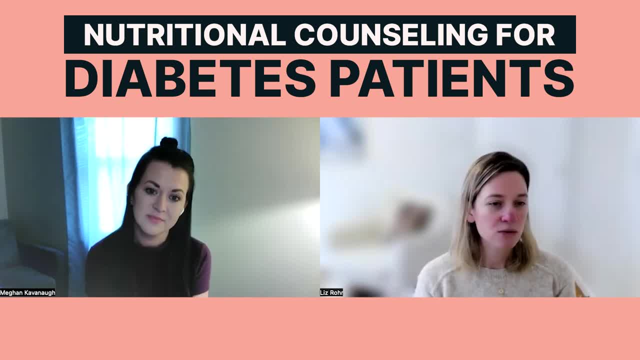 one of the ways potentially we can do this is: like how can we like? how can we like, how can we we can do it in primary care, like it's not against the rules to have somebody follow up in in a week- well, probably not a week, depending on how much space you have in your schedule, but like in three. 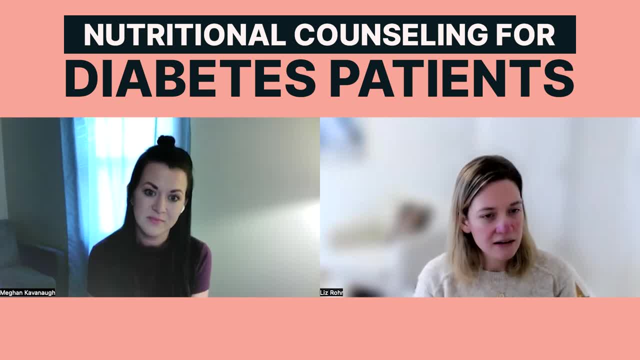 months if you fall, I don't. how often do you follow up with people in nutrition, like every month or every two months on their insurance? because, um you know, with medicare guidelines, medicare will cover reimbursement for registered dietitian for um nutrition or mnt, medical nutrition therapy. 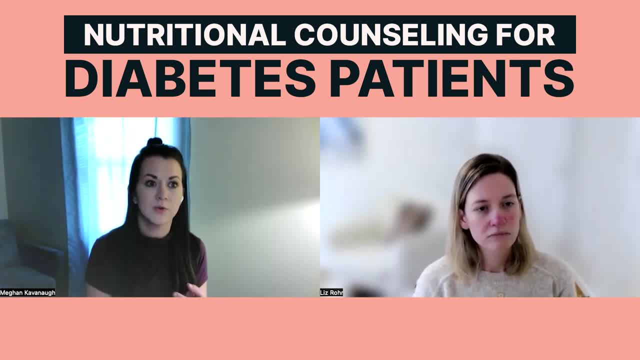 for diabetes and then for renal. so for your patients who go to dialysis, there's um rd on staff and then they get nutrition counseling, you know, while um at dialysis. so there's a certain amount, you get a certain amount of hours- and I should have looked this up because I don't think it's changed- but um certain amount of hours of. 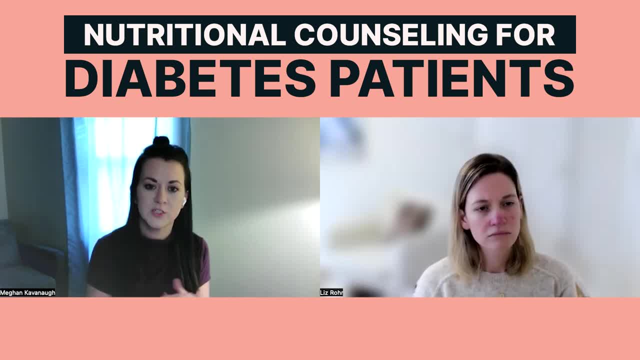 like initial mnt, like so the first time that they meet with a registered dietitian, and then a certain amount of follow-up. there's also um each year they're allowed to get kind of like refreshers, so it it does kind of depend, like so medicare, keep that in mind. 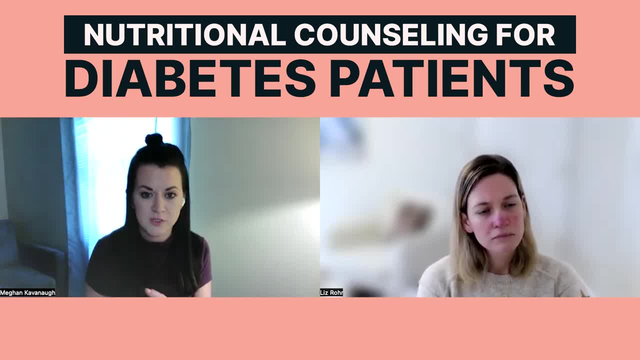 um. there are also a decent amount of private insurance company like blue cross um that will allow like a certain amount of mnt time, of course subject to like deductible and um copay and everything. so it just kind of depends on on how much support is needed and when um especially at 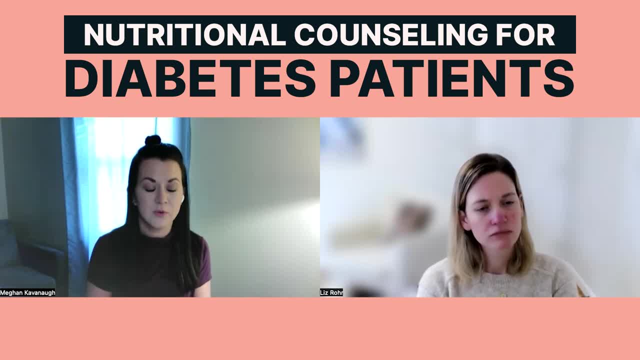 first, when somebody's newly diagnosed and you're trying to teach these things for, from an rd perspective, if you have the capability to have a pretty close follow-up- even three, four weeks, months, six months- and then you're able to get that support, and then you're able to get that support. 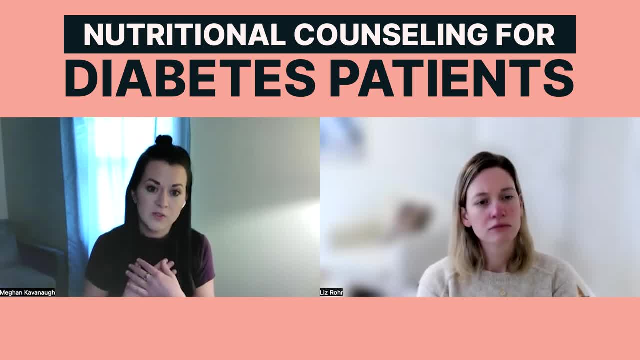 something like that, where they keep I- I like food blogs like I. I think that's very helpful. it's not only for like from my perspective of like some cause and effect, especially when I look at like some more detailed insulin management, but also when the patient is thinking through. 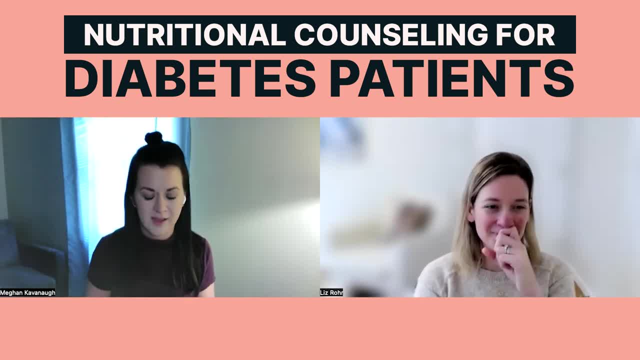 I'm gonna have to write that down, like I have to write down that I had, you know, some oreos for a snack and and you present this, if you decide to do this with your patient, because the day data is not just great for you but it's a really great eye-opener. 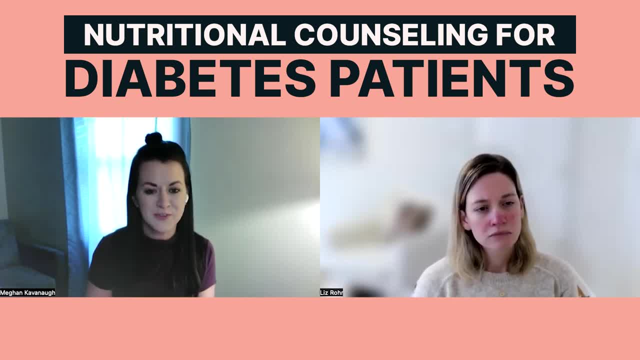 for that person, especially when you catch them, when they're motivated, like not, I don't use scare, like fear is a scare tactic, but a new diagnosis, like I'm going to change all the things, and so they're motivated and they want some feedback. and you know, as humans, we like positive. 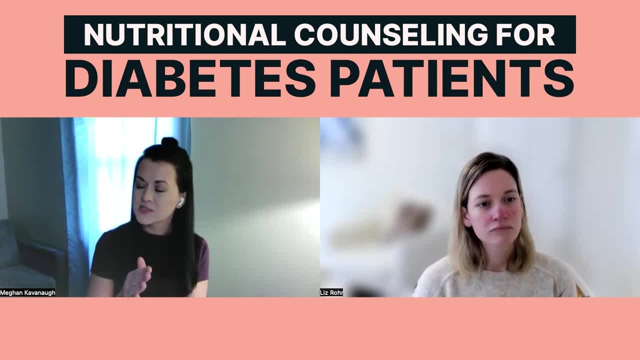 feedback, but telling that person this is not to grade you, this is not to judge you, this is not to like grade your papers. I just kind of need to see what's normal for you, like, hey, you know what, if you go fast, you're not going to be able to do this. you're not going to be able to do this, you're. 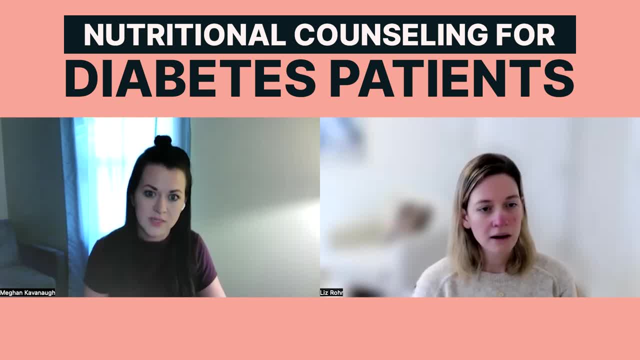 going to work on that. we're going to cut it back some, you know, and that's going to save you money too, like you'll see a higher, you know- account balance at the bank because you're not spending ten dollars every time. so finding that of it's not a, it's not something to use against them, you know. 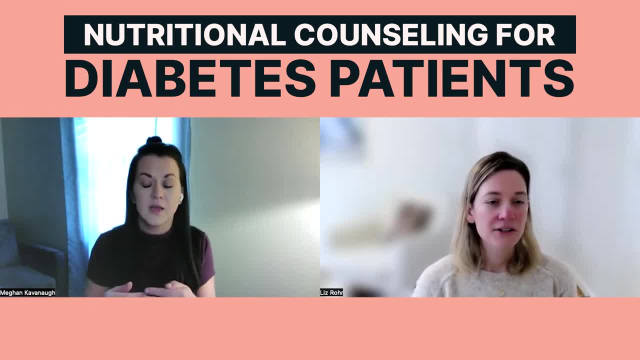 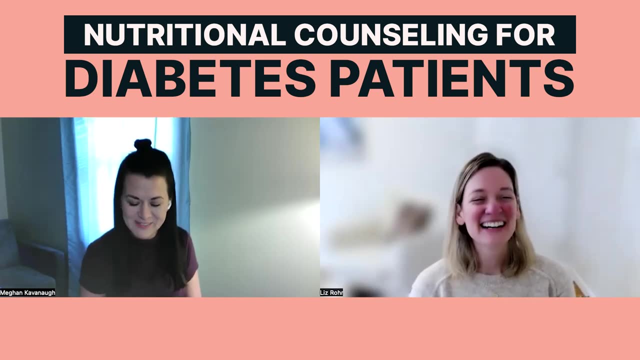 because, again, food being emotional. yeah, you're so right. yeah, yeah, it can be kind of an embarrassing thing like, oh wow, I really drink like four sodas a day, like this is bad, like they're going to fuss at me just to help. let me help you. I love that you brought that up because 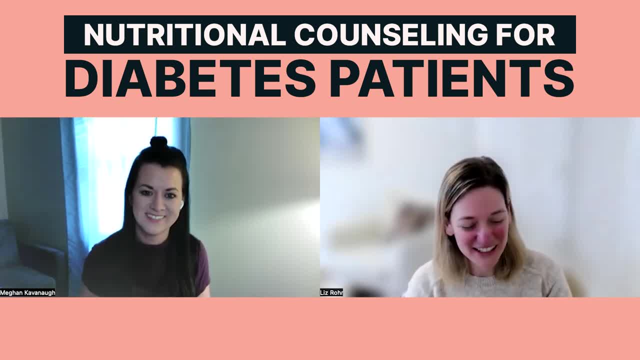 in a part that we're not going to include. I was- I was potentially offering to be your, your example patient, and even I, as a nurse practitioner, try my very best to be healthy. I'm like, oh, I don't know if I want the whole world knowing my dietary is right, and like it feels that same magnitude for. 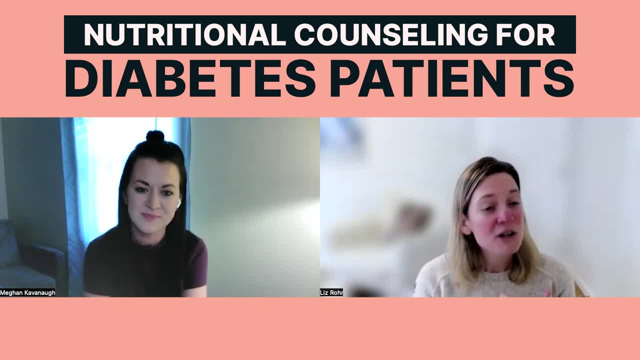 a patient in a clinic, especially if they write it down, especially they have to give it back, especially if you have that emotional eating components, right of like. there's a lot of feels in there, so I love that. oh yeah, I'm at this desk right now and it's like I wonder how many people would be like, oh my goodness, she's drinking diet. 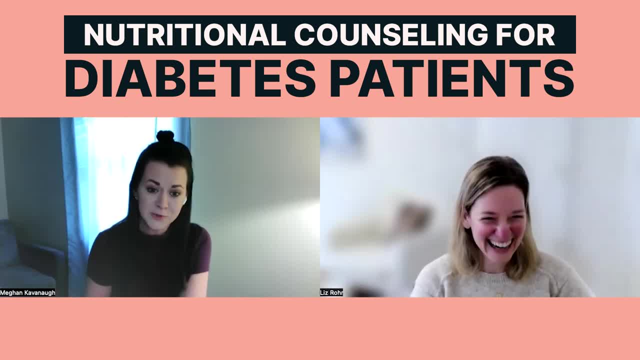 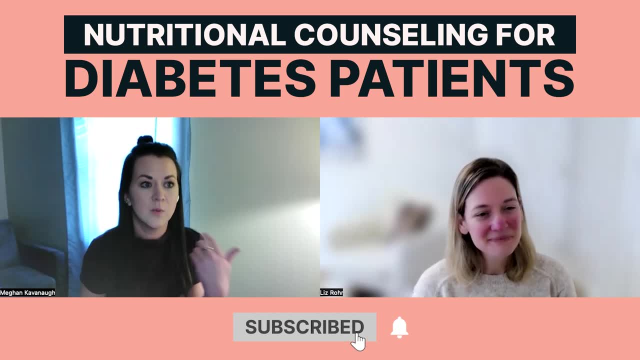 coke that has so many chemicals, but it gives me caffeine and I enjoy it. I drink a lot of water, like there's worse things, and I talk to my patients about that because they'll say: well, I don't want to do, I would rather have regular sodas, because at least I'm getting like real sugar and then not. 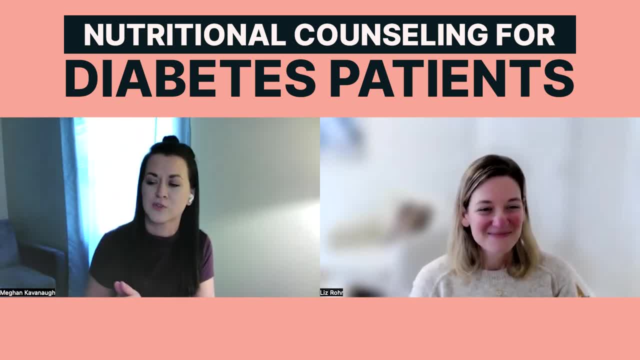 having like the aspartame or you know whatever other artificial sweetener. it's like: yeah, but if we look at like the hierarchy of like what's healthy, what's not, it's health promoting versus like health neutral versus health harming. like yes, I usually have a diet coke on my desk but I'm also flushing it with a. 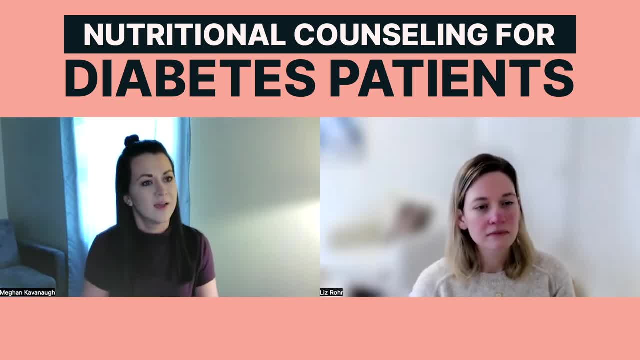 lot of water so I can't say don't drink them if I'm doing it and so you know. just things of just letting them kind of realize that you're a person too and you know your real world too, yeah, absolutely, and I really like I think, especially for newer grads, I remember feeling like I was like 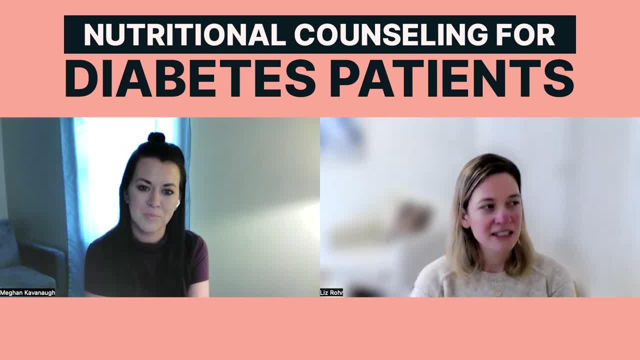 this way myself of like I felt like such an imposter and I was like I just like I need to prove myself, even to the patients, where they're like gonna think I'm an idiot all the time, like if you're feeling like that, that's super normal. and also, the more experience that I have, the more 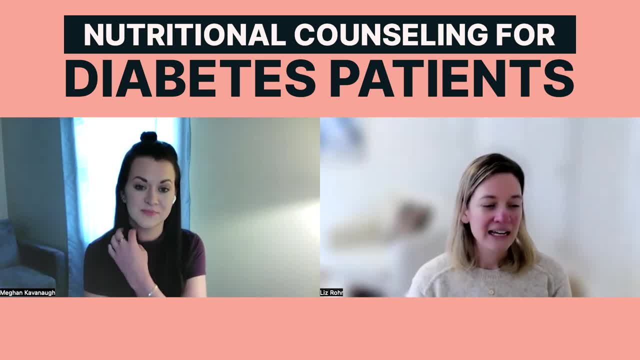 comfortable I am with saying things like I don't know, the more comfortable I am with sharing my own humanity because, like it's not, it's coming from a place that I'm just sharing, it's not like you need to, like you know, I'm not like putting it on my patient but at the same time, like when 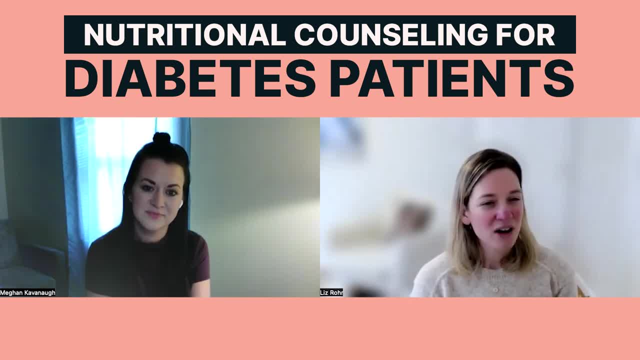 you share that you're a human too. like it's, people are going to feel more comfortable with it, and I'm more comfortable. I want to. I want to go back to what you said. I guess like a couple of what I'm trying to tease out is: like it's, it's. it sounds like you know we need to do like one thing: that. 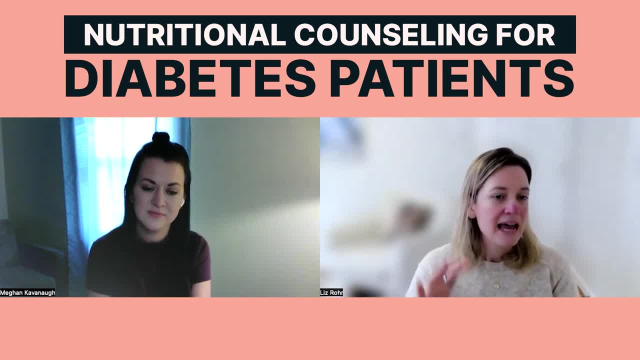 one opportunity is that we could do more assessment, questions and asking and really getting a sense in a deeper way of how people are actually eating on a regular basis, not having any judgment about it. we can do our own follow-up visits as primary care, as a count health dietary. 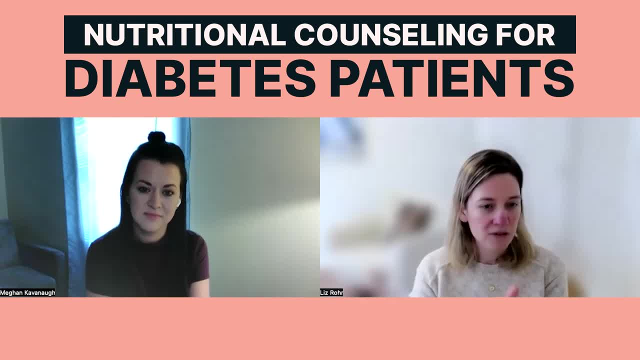 counseling visit. right, it could be a diabetes related follow-up, for example. and we can have these conversations. I'm not, I don't have the skill that you do as a registered- you know- dietician, but at the same time I can do my best, and then you know. just another recap. 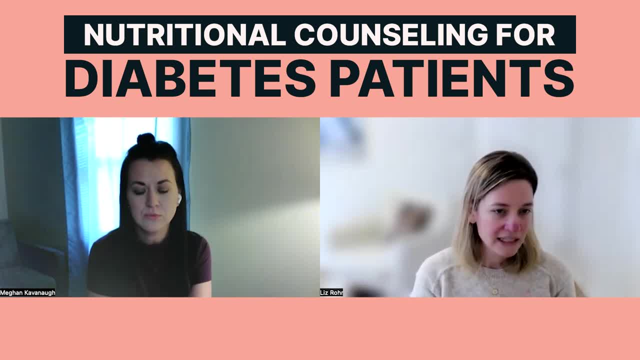 thinking about high glycemic foods and low, lower glycemic foods and potentially considering substitutions as like one like quote-unquote hack- it's not really a hack, but like what is one? like small change and what are some of the other like? when you said: making the best choices in the 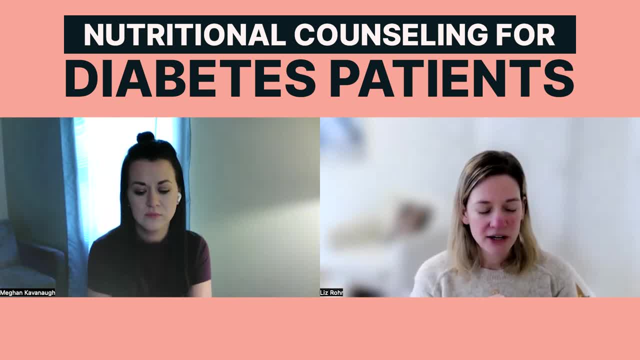 moment, like what are some example? or if you can recap what you shared about the best choices in the moment, like what are some examples that you give for patients of like how to make their best choices, whether it's like a fast food like here are the healthiest options at this fast food place? 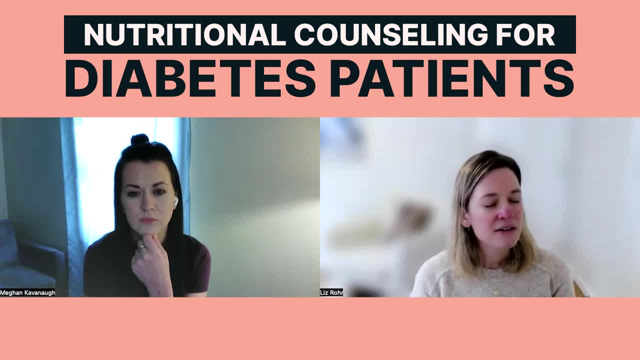 versus is a smaller portion size. do you know what I mean? like what are some? can you think of any other examples of of patients: where you're, you're, how, what is their guidance of making the best choice in the moment? so if it's more of a situation that's um, let's say, social, like family gathering. 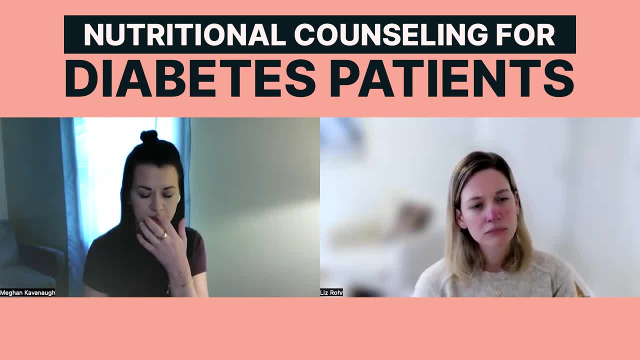 and you know potluck style something you know where. there's going to be quite a few different dishes I'll encourage, hey, you know you be in charge of something that's healthy, that you know, that you enjoy, that you get joy from. that is going to promote some well wellness and not just 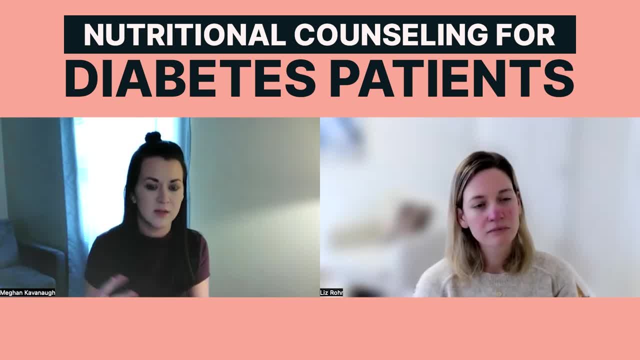 shoot your sugar. so if you know that, hey, this salad that I make with this salad dressing that I enjoy, I like the way it tastes, I enjoy it- other people would benefit from it too. so you know, you kind of have a food going into it that's kind of safe for you and not so much like a. we call it a. 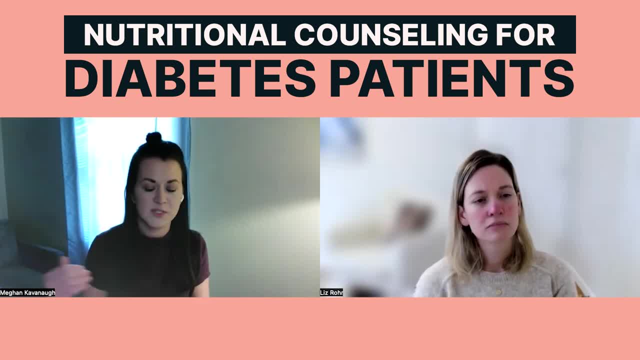 trigger food. so, um, if there's like tons of different types of starches, which a lot of times in those social situations there are okay, like you're gonna have some, but what? what are your favorites? okay, so let's think about thanksgiving. we just had thanksgiving a couple. 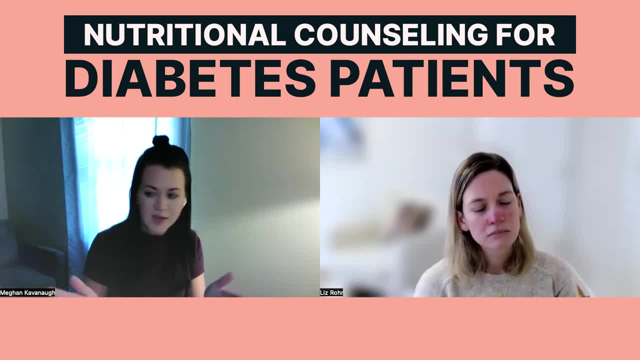 months ago and I love asking the patients. it's like coming back, how's the holidays, like what's going on, like what was the best thing you ate? tell me the best thing you ate- and I do this right now, so not as an arty, and you know- and like, oh, I love that. so we're bringing some positivity around food. 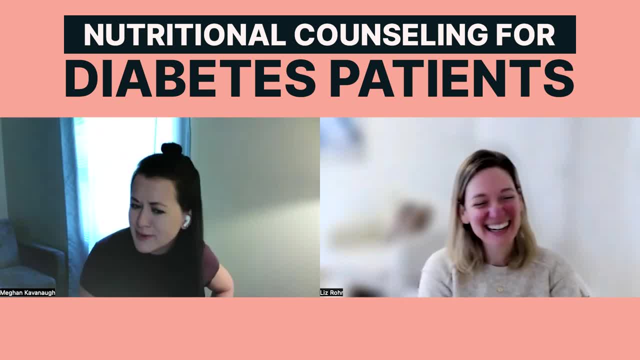 just like, oh my gosh, I did a bad job over the holidays. like: how much pumpkin pie did you have? it's, yeah, non-judgmental at all. and then you get that comfort level like that from them, because it's hard to talk about food and again it can be embarrassing, um, for some people, but so because 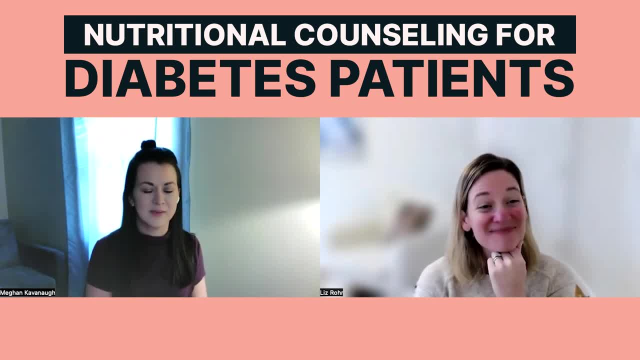 if they don't want to say, oh, I don't know, you know I cheated, I was bad. and I don't like when people say they cheat and they're bad, like no, you're human, you are human. so dressing that's my thing, dressing like I don't care about stuffing for the northern. 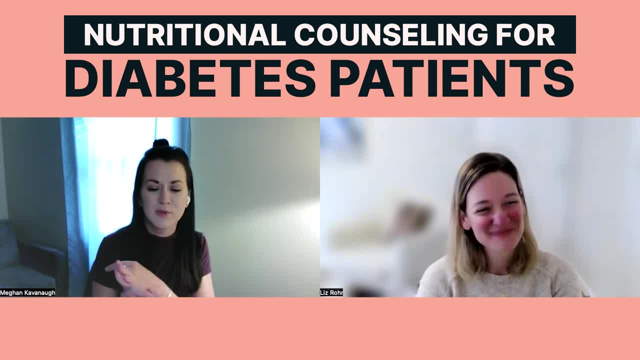 yeah, my mom's dressing or my mother-in-law's dressing, like give me a pile of that and some turkey and like I'm good. so then they'll. they'll say, oh yeah, that was my favorite too. and I'll say, because I don't really like, this is me, you know, talking. I'm using myself as a patient, how about? 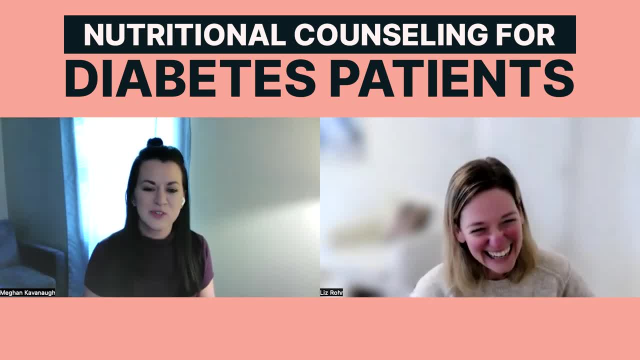 that Liz instead like I don't really care for like uh, seasonal dessert like pecan pie and pumpkin pie and stuff. so I'll tell the patient like yeah, I don't like that stuff, but I'm gonna eat some dressing and I'm gonna enjoy it because I can only get it this time of the year. 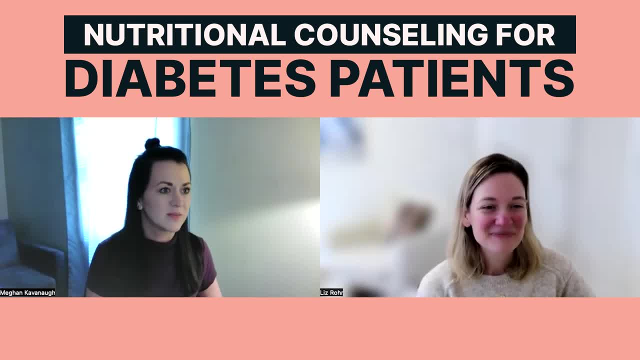 what did you like? you know a lot of times like, oh yeah, it's my aunt's sweet potato casserole and I had that, but I did good because I ate some extra turkey and I didn't have that. it's an accomplishment. so those types of things and environments, because we are going to have. 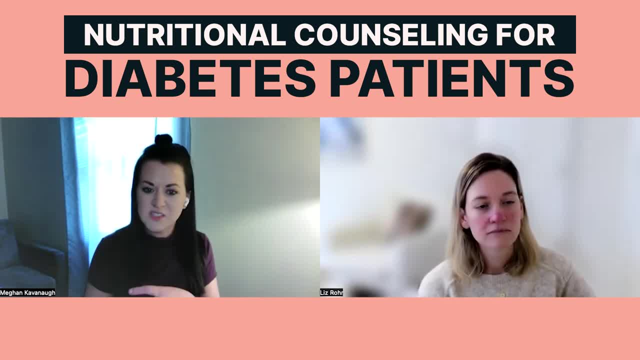 holidays. we're going to have birthdays, we're going to have events at schools and you know there's going to be things. so you is, when we're talking about like how difficult it is to say everybody gets the plate method or everybody we're going to hand. 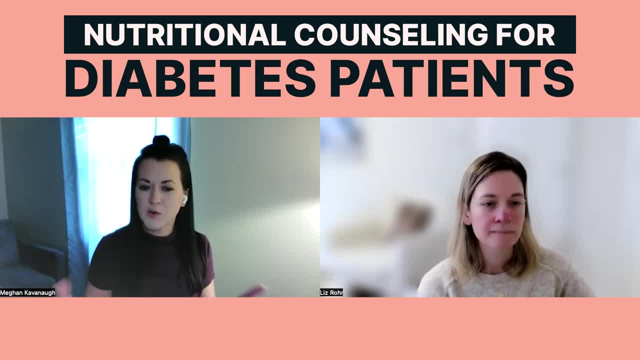 hand out Mediterranean, hand out keto or whatever. that's not real world a lot of times. so it might be having. okay, I really want to enjoy this piece of birthday cake, but I'm not going to have ice cream on top of it. but that doesn't mean eat double the cake either, you know. but, um, when it. 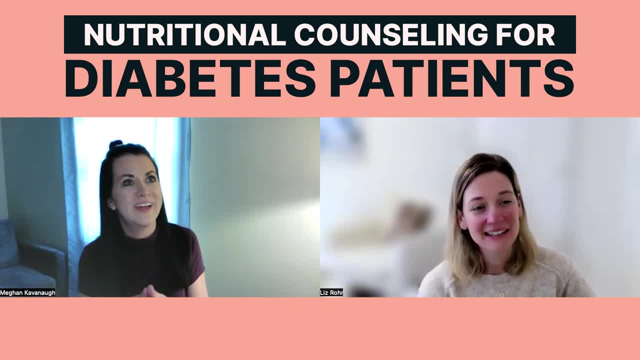 comes to. that's a long answer for your short question. oh, it's great. it's like these little tangible things and they remember that. they remember like I went and saw Megan and she was just saying like if you don't like something or you can get it any other time, you can get it any other time. 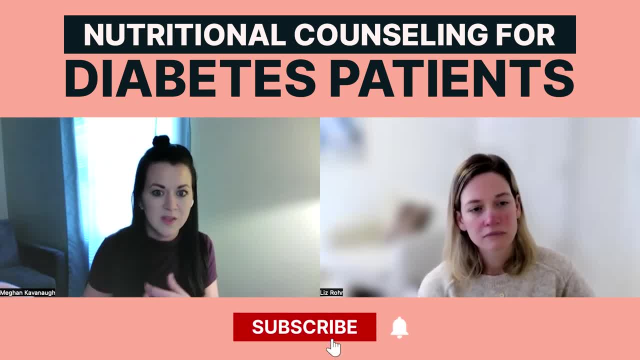 at the year. why kind of like waste something on that? you know being like a special food, yeah, so when it comes to restaurants, um, and fast foods places, now most, most chains have their information online. okay, and I used you know it's easy. but I know the easy thing to think about is like: okay, 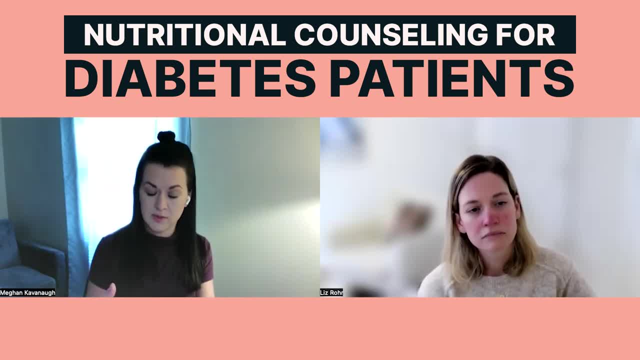 if you go and you sit down somewhere, think of it as the plate method and, for people who aren't that familiar: half plate vegetable, quarter plate protein, quarter plate starch- okay, so quarter plate of something that could possibly raise blood sugar. most places that you sit down at have a lean-ish protein option, a starch and then a. 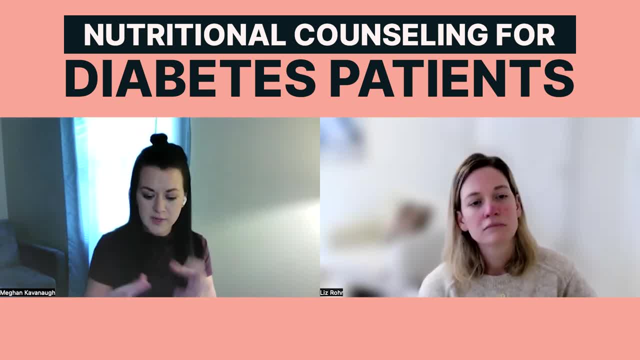 non-starchy vegetable or salad. so it's like if you think of that plate as the platter that they're going to give you in this huge portion, that's, that's a win. just you know if you usually get a giant plate of pasta but the healthier option is to get a protein vegetable and a small amount. 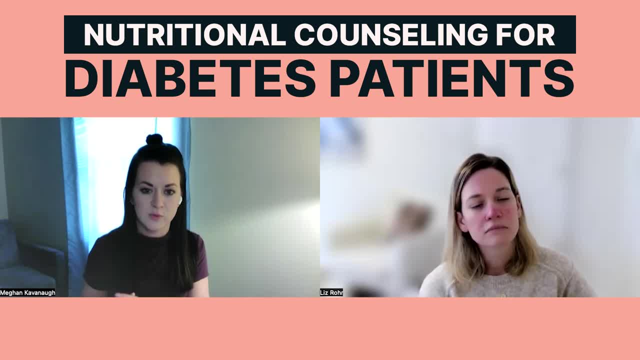 of a carbohydrate. that's a win, you know. that's a great, great improvement with, at the same restaurant, somewhere you enjoy, if it's date night or whatever. and then kind of the same thing with fast food restaurants, if it's somebody that's traveling and, um, you know, they just didn't pack something or because 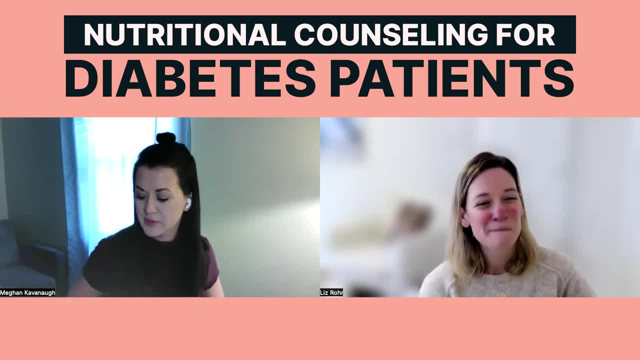 that would be, you know this ideal world that we would say: but um, people would pack all their stuff. but that doesn't happen. and so, okay, if you run through mcdonald's, look at the menu, kind of, look at the carbohydrates, look at the different amount of carbohydrates and, um, you know the. 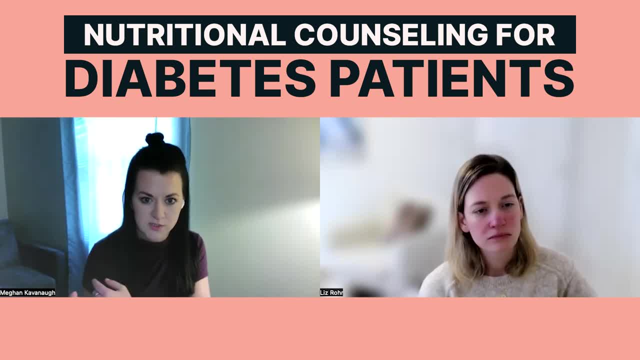 amount of grains and grains you're going to need. it's a lot of carbs and you know the things that are going to be walled up in this menu. you can't kind of tell why there's so much of you know in a large portion of this area and you're going to be watching like, oh, i've got more carbs, i've 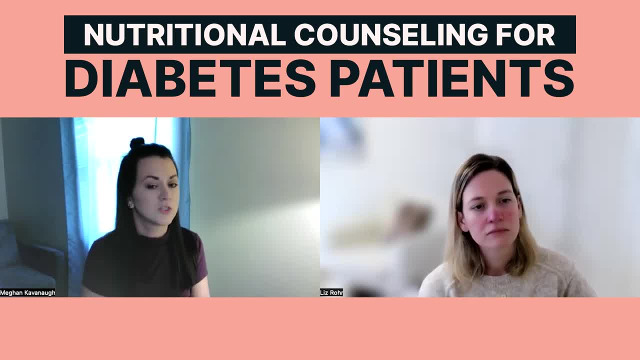 got less carbs now and i'm going to have more carbohydrates. i'm going to have less carbs, i'm going to have more, you know, and that's a big one. um, i don't think it's a big difference between jessica's and mcdonald's. i mean, it's very different. um, i think it's a very different. 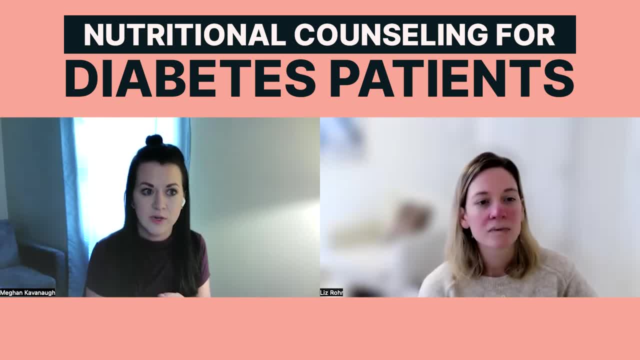 you know, it's like they have a little side salad or they have, you know, apple slices or something, but it's just automatically tailored down and most of the times it's satisfying enough. um, we're kind of taught over time to not really think about satiety and eat past the point of fullness, and 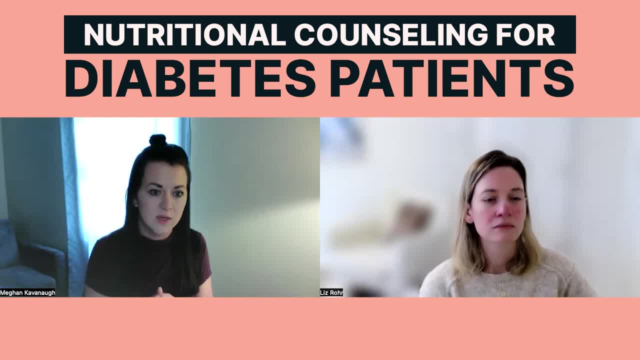 or don't waste things that are on your plate, because you know you're just kind of pushed if you were kind of that generation. so people don't even really recognize when they're actually satisfied versus like stuff to the brim and then feeling sick. so you know, just then you start. 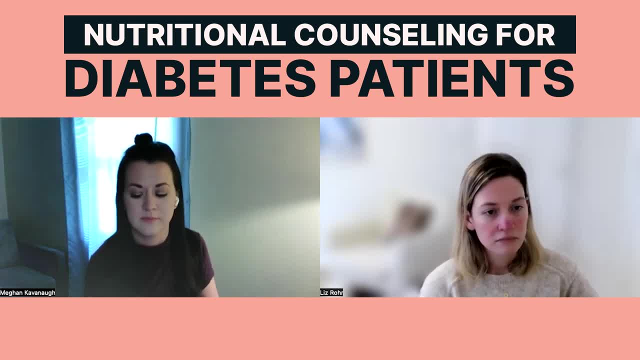 getting into more intuitive eating too, which, like everything else, takes a lot of time. yeah, absolutely, absolutely. it kind of reminds me of like when i talk with parents: um, do you see kids? i can't remember, do you see? uh, yeah, um, but like with kids, like when we talk, when i talk with 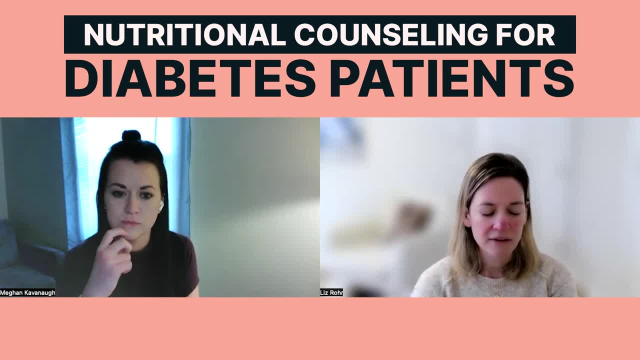 parents about, um, uh, or the caregivers of young children, like about picky eating, and it's kind of like- and obviously i would love your take on this too, but i, with the way i talk about it with them, is kind of like, um, there's a lot of drama that gets created between you know, there's a power dynamic and 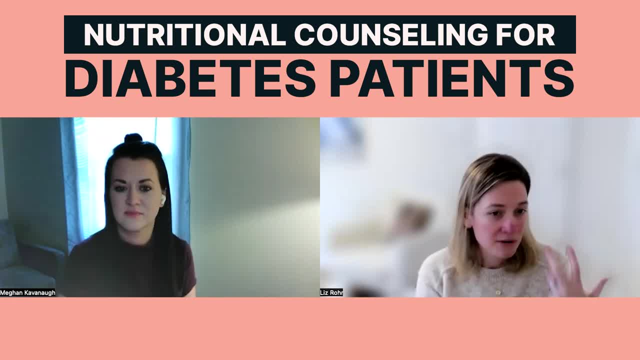 kids can only control certain things, and that's one of the things is like what comes in and what goes out of their body, basically, um, and so it's like you can, if you can remove, like to put, try your best as the grown-up to like, put your patience, like, work on the patience of like. 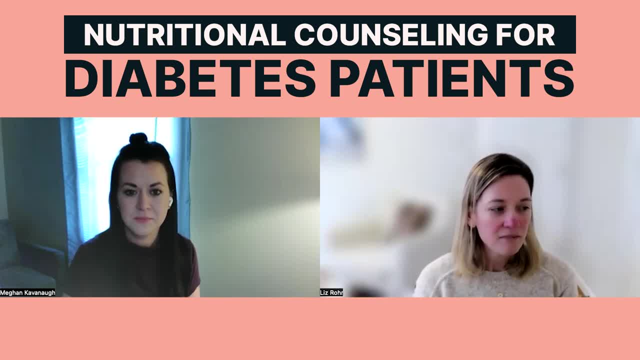 letting all the drama be out of it, letting all the feelings be out of it and also trusting your child to know they're like. it can be a process, since every kid is a little bit different, but it's like the. the main goal that i talk about with parents is like how to encourage your child to be aware of when. 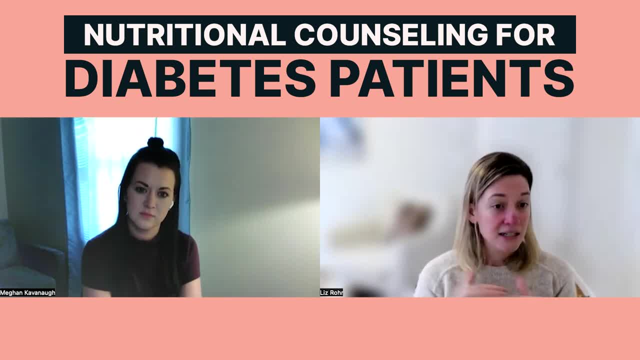 they're hungry and when they're full and like allowing themselves to be done because, um, and obviously you have some behavioral stuff in there where somebody will eat like a bite of something and then, like before bedtime, they're like i need to eat this whole thing, right, but it's like even. 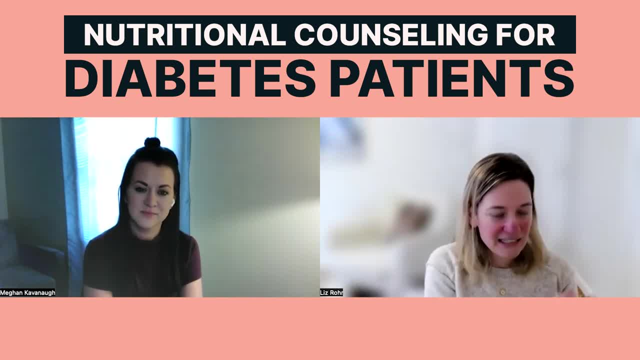 with adults like i know that that's it's. it's easier when, when kids like that, they start off with that. but like, even as adults, like we can have conversations about that. of like thinking through those pieces too, of like you know, like do you know when you're. 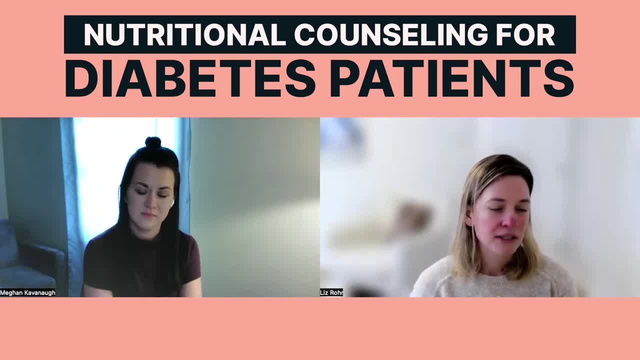 full. do you know when you're hungry, like what are some things to practice around there too? yeah, and what does that feel like? are you? like, how quickly are you eating? like, are you, are you a nurse at the hospital and you have to eat in just a couple minutes just for literally to get? 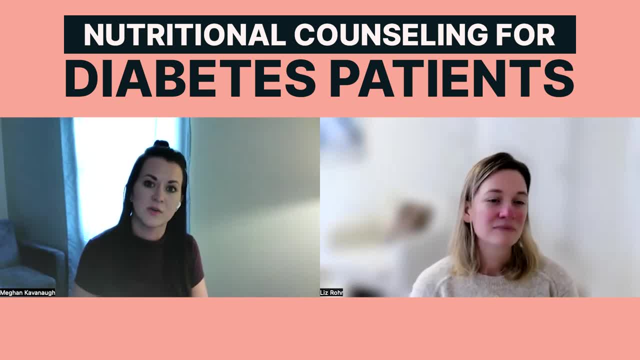 calories in your body to and get some sort of nutrition. so and and yeah, i mean that's. i would say that's very challenging to teach- um like knowing, like hunger cues, and then you know, since we're talking about diabetes and with like weight management, you know these, the glp ones. yeah, that's one of the things that's so helpful. i mean, then, when these 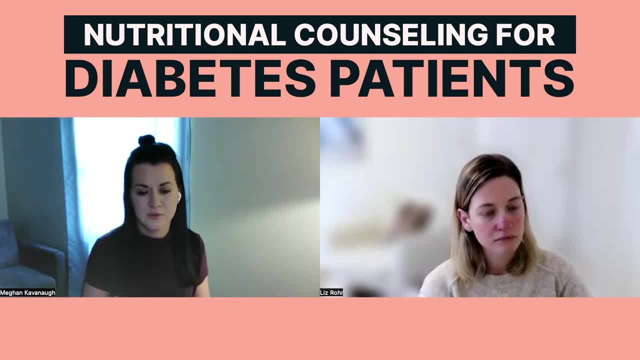 um, patients come back and i i told you before, like we started, i was like i really don't want to get into like weight loss, yeah, yeah. but i'm gonna kind of dip into it a little bit like from the diabetes perspective, when you've had somebody that has struggled with weight management and 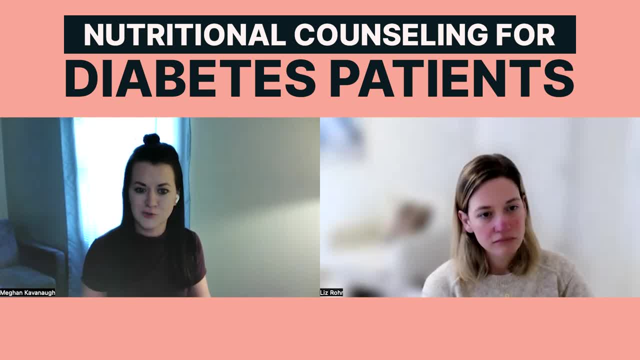 you know, because obesity is not being treated with it. it's just it's kind of a problem in and of itself, with kind of limitations on medications and insurance coverage and everything without diabetes. but we know that it can help prevent diabetes and so if you have somebody that's been told their whole life, you know that, like, your bmi is too high and you're 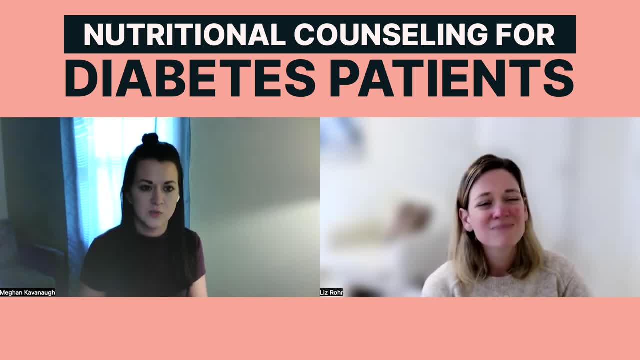 overweight and you know this, and there's such a negative connotation with food and then you have one of these medications that all of a sudden, when patients come up- i'm not obsessed about food, you know, like it's, it's great like i can get halfway through my meal and i'm like i'm good, like i've 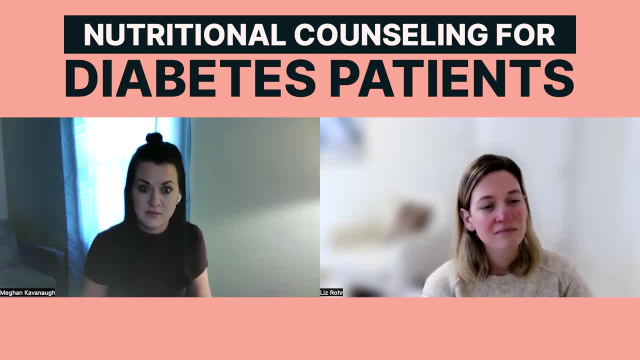 never had that ability to be able to, to stop or to realize that, wow, i really am not that hungry and i don't need to snack four or five times a day and, um, and, in that regard, kind of have that because the medication makes you full or, you know, it makes you feel fuller longer. yeah, amongst other ways of 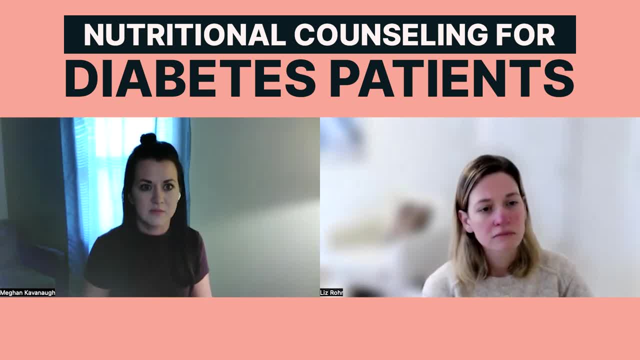 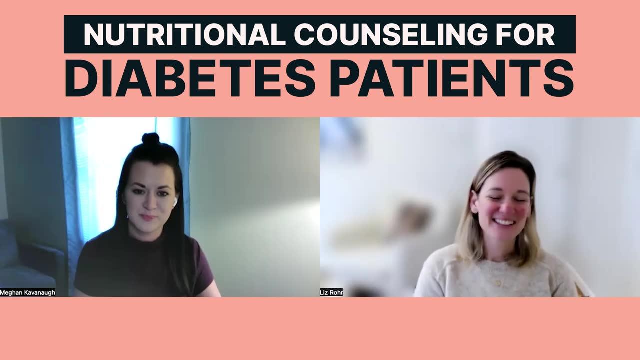 just how it kind of shifts the brain and creates a lot of like positivity emotionally too, because there's not as much of a obsession with um, like snacking and binging and things like that. but that goes totally down another rabbit hole totally. oh my goodness. oh my goodness, you're so right. one of the questions i really love that was submitted. 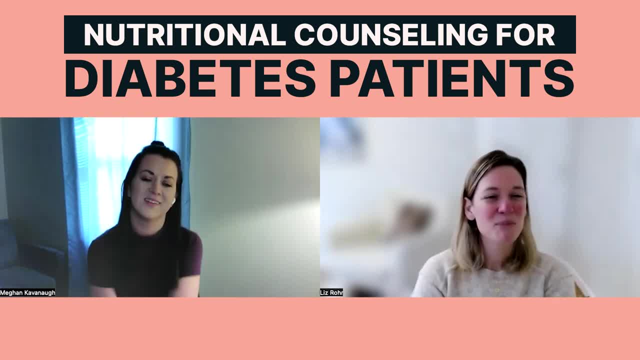 was: um, what have you counseled patients on? that they seem most surprised to hear. is anything coming to mind with that in regards to foods in general? yeah, just like. i guess like when you are working as an rd and you had a patient come to you and you started counseling them. 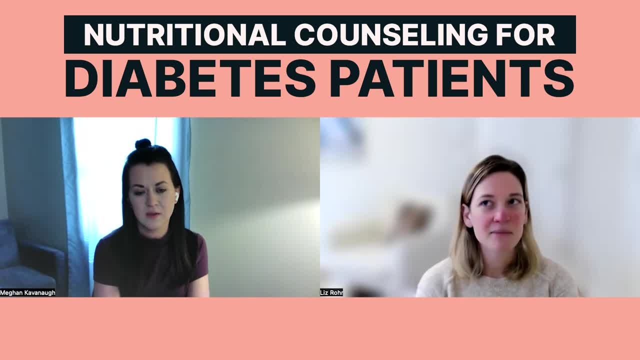 and they were like really surprised. are there any themes that came up like like, um, um. i feel like, for example, like when i would uh take care of patients in the hospital with ckd- um pretty late stage ckd- and we would be serving meals and we'd be talking about potassium in. 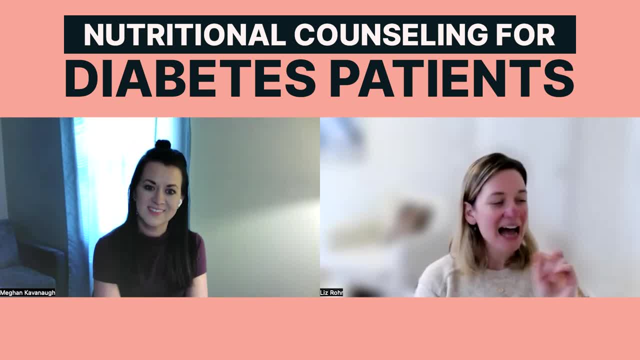 milk products and i'm like, really i'm like tomato saw, like wait, i can't have milk and i can't have tomato sauce. right, like i can't have milk and i can't have tomato sauce and i can't have milk. and like like we had more conversations that. but do you know what i mean? was there anything that like? 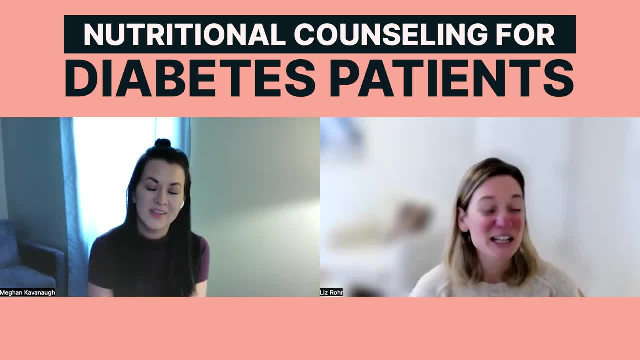 currently comes up that people are like really- because we probably would feel that way too in primary care- being like, oh, shoot, so with diabetes management and when we talk about starting with foods and, of course, like the focal point being like carbohydrates, it's really rare that anybody 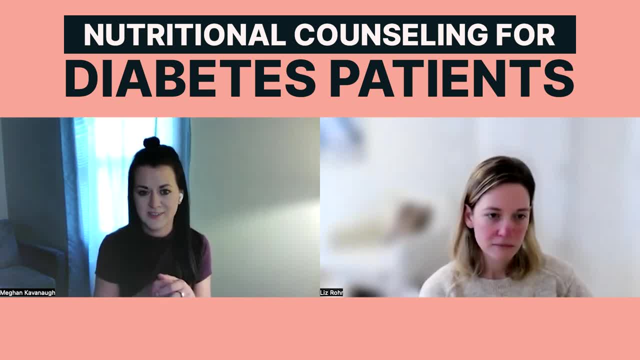 talks about, like the blood sugar changes that happen with fat and protein, yeah, or even low, like even very, very low carbohydrate vegetables, like you know, green beans, broccoli, um, cabbage, all that- but really you don't see that unless somebody's wearing a cgm or they just kind of have. 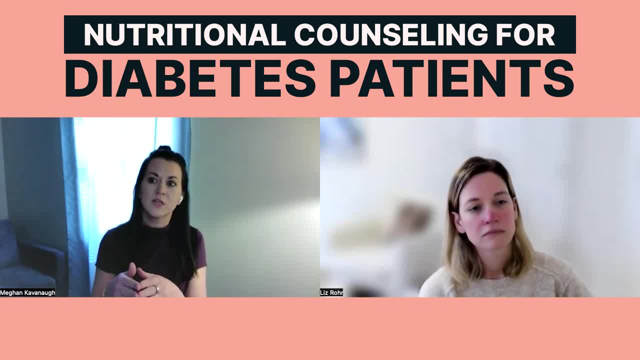 to um check their blood sugar a little bit more often. so if you have somebody that is still, you know, going pretty low carbohydrate, or if they have kind of a lean and green meal and you're watching a cgm and you're pointed out to them and maybe it's like a higher fat um steak or you know. 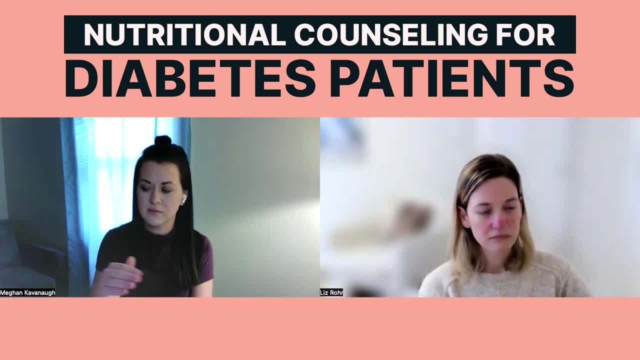 or if there's a lot of oil on something, and then it's like this late little rise and it's not an aggressive rise, but like what is that? they didn't have any carbohydrates at that, at that meal, and where you can see that where some of the protein and the fat. well, you'll still have a response. it's. 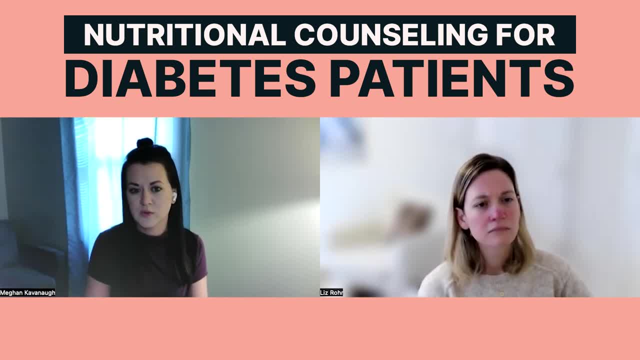 not an aggressive surge but i would say that's a big surpriser for a lot of people and when you look at like insulin management with that- especially if somebody's wearing an insulin pump, there's different tricks that we can use to kind of combat that like a post meal. 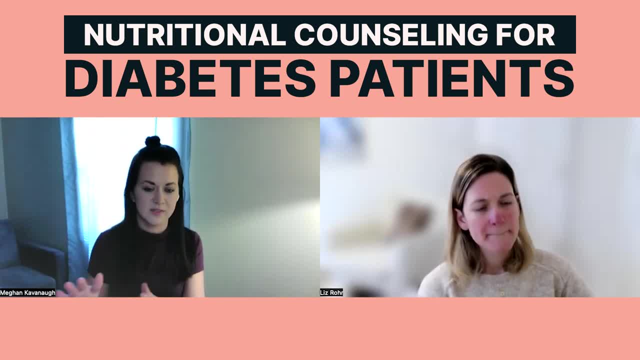 bolus based off the amount of protein and fats, um, and they can combat that without just waiting to go high and like get a correction to come back down. another really big surpriser for um, blood sugar spikes- for not everybody, but we see it a decent amount, especially if they're wearing a cgm. 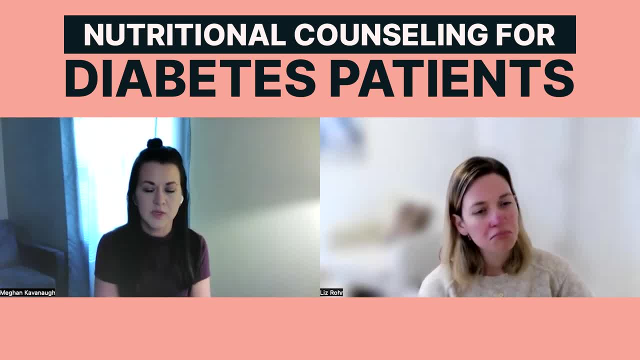 is coffee. you know caffeine, like anything, that's a stimulant. so they'll wake up cruising really good and then even if they just have like a black cup of coffee and it's 100 milligrams of caffeine and that stimulant you see that like go up. so there's a lot of times that we have to teach that patient this is getting. 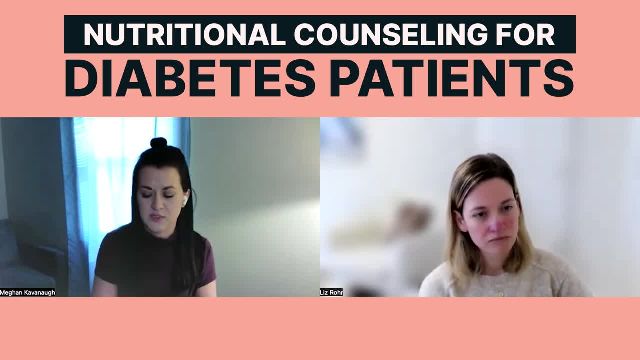 into type one and like insulin dosing or type two, like resistant on insulin, where they have to input some carbohydrates for that, because we see the response to get ahead of the spike. because it's one of those things that even though it might be zero calories, if there's no sugar, no cream for in. 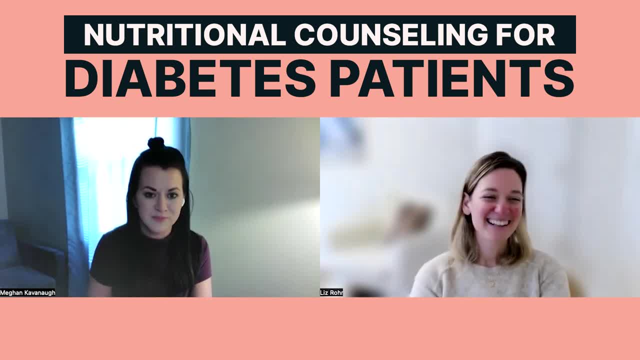 it, it still can cause a blood sugar response to it. oh my god, that's so fascinating kind of some of the like non-obvious things that you can see that are going on in the blood sugar response to it. yeah, really interesting with time. yeah, yeah, and do you see that with other caffeine related? 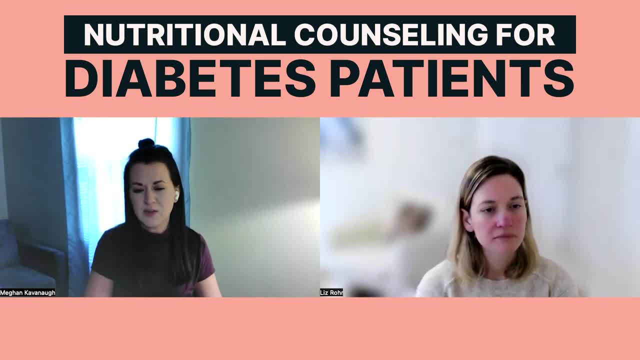 products like tea or energy drinks. yeah, tea i don't see quite as much, unless it's like a really large quantity of like ice tea. so i do have some that, uh, even with unsweetened tea and, um, not even putting like an artificial sweetener, because you know there's that kind of that potential that. 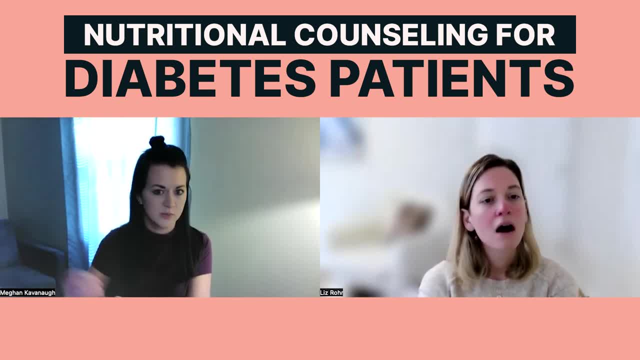 artificial sweeteners. like the body can't distinguish a difference, there might still be a little blood sugar response. so that's kind of. but even unsweetened tea in a large quantities you can see it. you can also see it with um nicotine. so for smokers you can, i think. 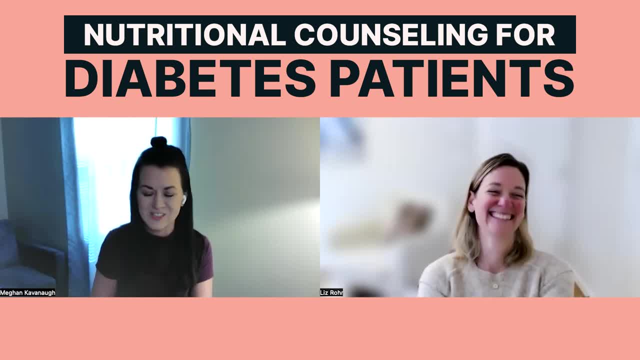 sometimes be like: is your smoke break at 2: 30 every afternoon and i see this little spike in there. but, um, those, um, those really high caffeinated- i can't remember some of the brands, but they'll be sugar-free like something like a red bull. you know, you can see it. yeah, you can see it there too. 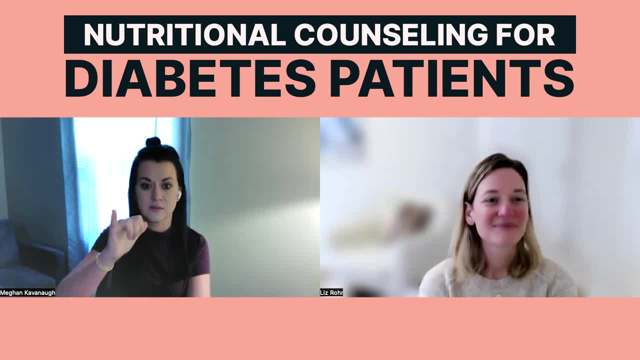 especially because a lot of those people don't sip. it's like a chug, get it back up and then go back to work. oh my goodness. well, this has been super, super helpful, um, and you said that there are some resources that you recommend and you and i can connect about that, um, in terms of like i mean. 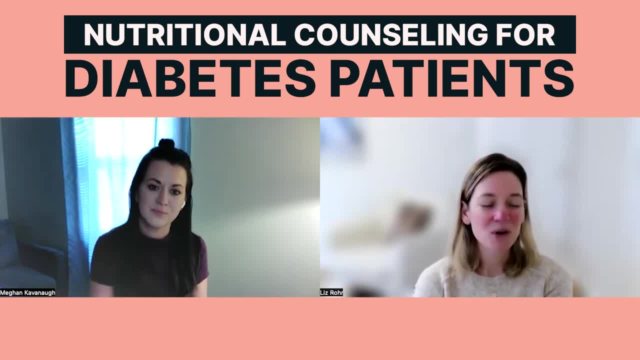 you have your own custom handouts. it sounds like- and and i think the sounds like- the moral of the story is that like it's really not about handouts, it's about more of a history taking and a customized approach and like thinking about what are those lifestyle changes we can make? what are 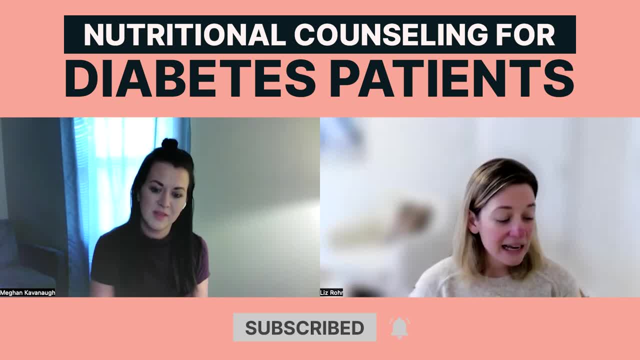 the lower glycemic options and, um, yeah, any other kind of like parting thoughts or pearls, or actually we didn't even touch on the, the difference between dietitian and nutritionist. do you want to? oh yeah, well, let me say one more thing about like getting a history, so just to. 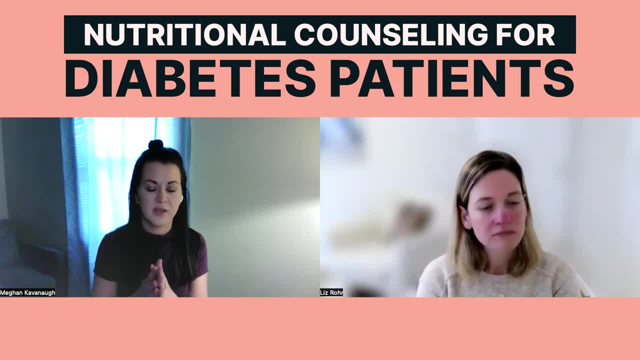 to be clear, like when we talk about getting a history and everything. those were visits and i don't know how a lot of rds are are scheduled like in our clinic, the first visit with the dietitian baseline is scheduled for one hour. yeah, so it's this, this type of education, this deep. 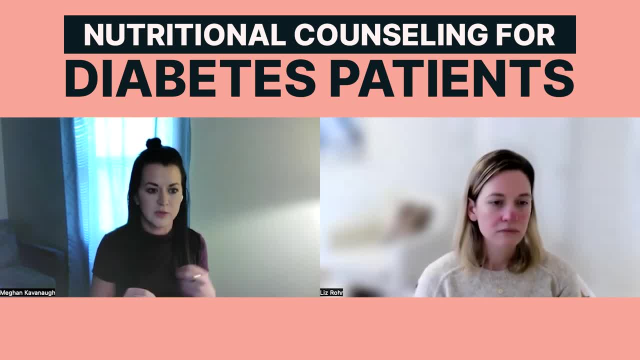 like the history, taking the recommendations, talking about it in response, like with medications and stuff, this is not a short process. so i'm sure some of your eyes be like i can't do that, like i can't even do what i need to do in a 15 or 20 minute spot, but and that's where you just give- 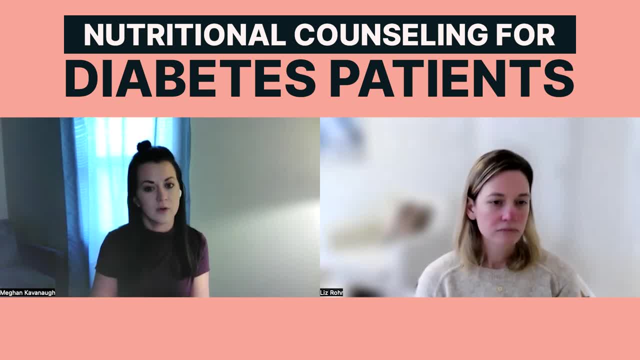 them like little bite-sized pieces of hey. at the beginning, we're going to work on no sugary drinks like that's what we're going to work on right now. then i want you to start looking at carbohydrates. maybe think of them as like in serving sizes and start reducing their increasing protein and 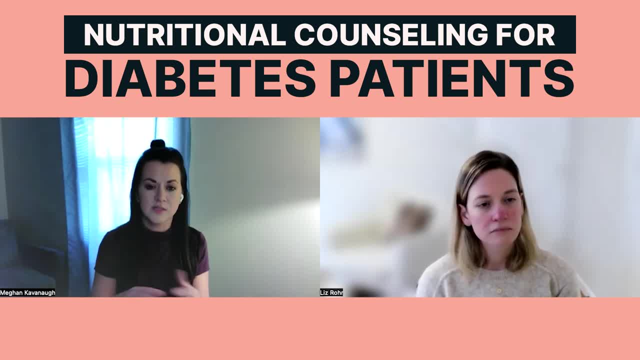 vegetables like that's what we're going to work on right now and then we're going to work on those, can be just like little basic things, as long as they have a concept of what you know carbohydrates, fats and proteins are. so these are concepts and conversations that take long periods. 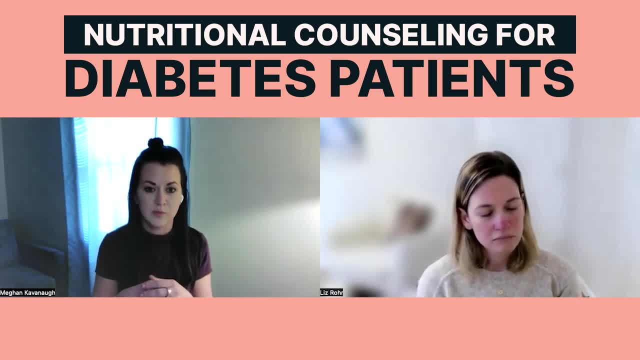 of time like there would be some my previous placement appointment that'd be more like weight management counseling. that would be hour and a half or two hours, i mean. so it's like huge, huge blocks of time to get the information and and have those really uh, deeper conversations totally well. 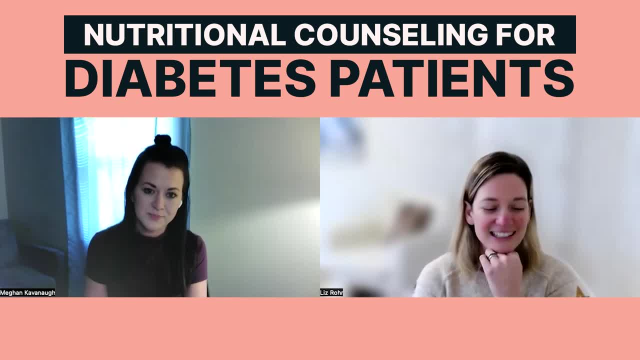 i think, yeah, no, i appreciate. i appreciate that reflection because i sometimes i can be overly ambitious. i'm like i'm gonna start doing that more. hold on, hold on um. but i think that also reminds me of um, uh, we have uh. at one of the clinics i worked out, we had a diabetes, um nurse educator and um, she had a. 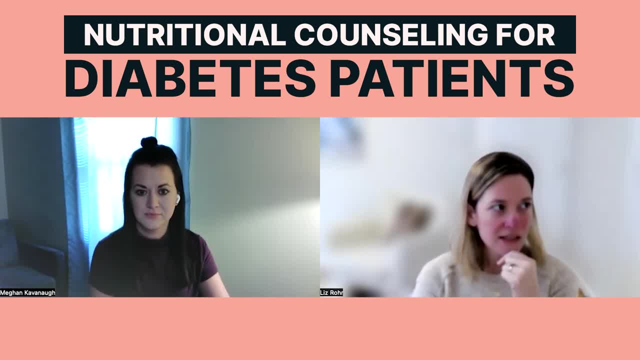 lot of time to work with patients and so, um, typically not that it's the best way to run. well, i'm not gonna split hairs there, but there are a lot of times with. the nurses that i've worked with have been really supportive, whether it's for hypertension care or diabetes care, and- and potentially that could be an. 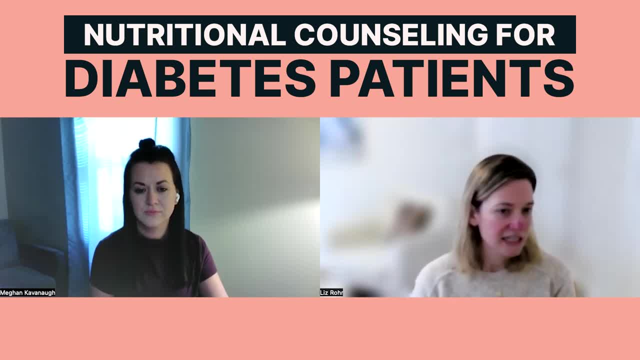 opportunity to partner with them. if we don't have the access to a registered dietitian of like, how can we partner together to have more time with the nurse, get information, and then we can kind of be, have it be a more time together in general between the two of us type of thing too, and and 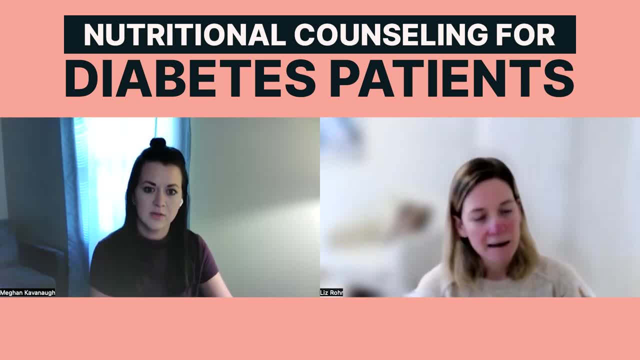 with things, that, how they change with, like telemedicine and telehealth and making sure, because not- and this goes into that other part of it, but i think it's a really important part of the question that you just asked about with dietitian, uh, nutritionists. so, um, with our national board. 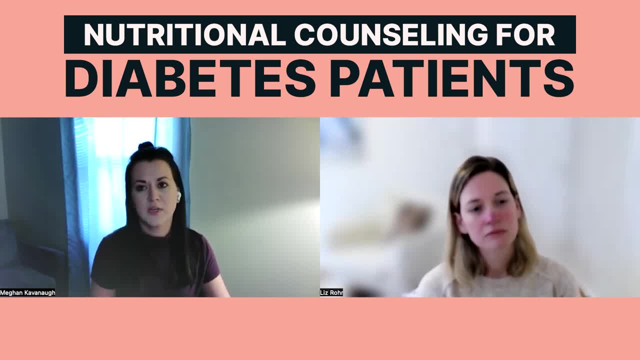 it's registered dietitian nutritionist so it's rdn. but not every state in the us has licensure. so in louisiana we have um a state board, you know, for licensure. so it's like title protection. so if somebody like even for like telemedicine, they have to be licensed in louisiana, of course you. 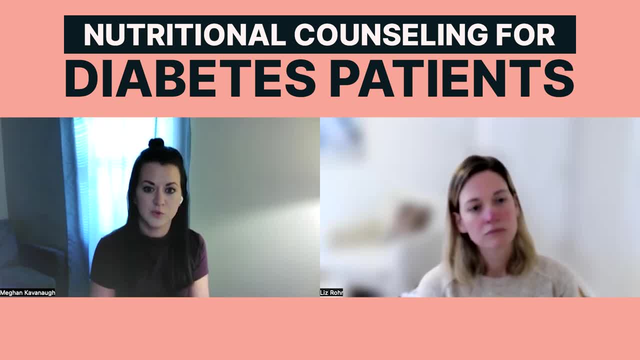 know, like anything else. so that is another option, if there's one- and i just did a little bit of quick research- the um, the eat rightorg, which is the um overarching for registered dietitians. there's a place to search, like in your area, for registered. 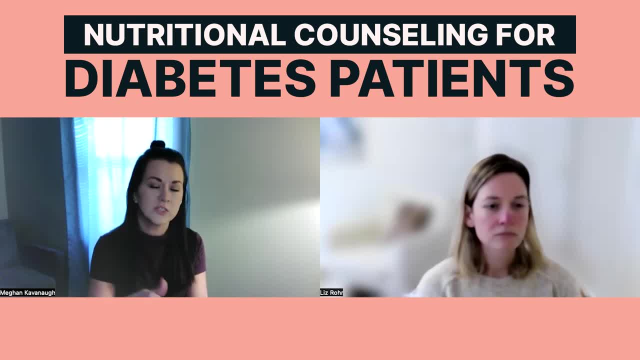 dietitians that do telemedicine, so, or just locally, or telemedicine and um. a lot of hospitals also have outpatient programs, so that that's another option too. just trying to find somebody that you can refer to. that's usually where i would say, that's where i would say, that's where i would say: 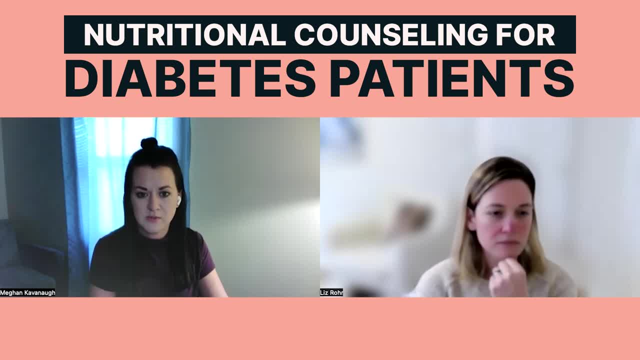 most places. yeah, yeah, yeah, and there also might be classes available as well, um, but don't don't forget that if telemed or telehealth is an option as well, i love that. yeah, so well, that was. i think that was the thing that you and i talked about before we ever worked together. the first time was: 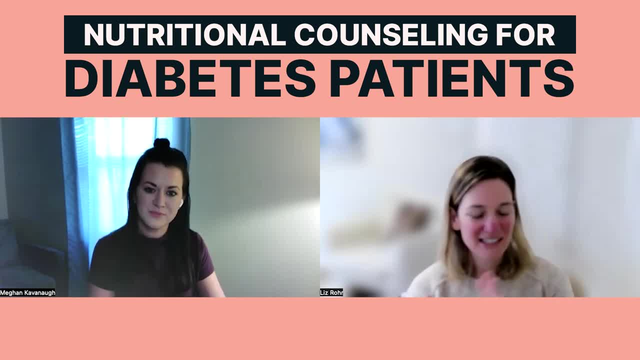 um that there's a difference. there's a dietitian, there's nutritionist. seems like everybody has different preferences for names, but the national one is rdn and every state by state may or may not have a licensure process, so somebody could be operating as a registered dietitian or a. 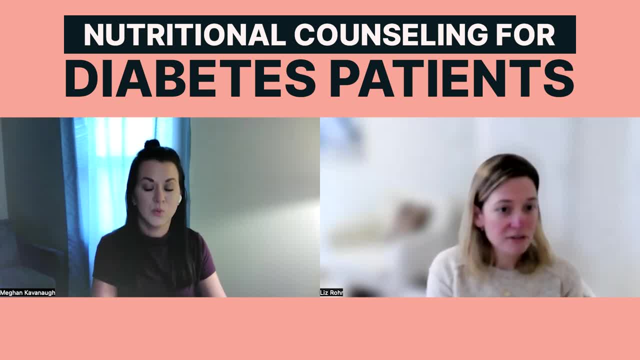 nutritionist but not actually have the certification credentials, right, right, yeah, or you know, because there's a, of course, now you know a lot of health coaches and i mean there's instagram influencers and stuff. so i mean, ideally you would have that, that person that has that four or five degree and 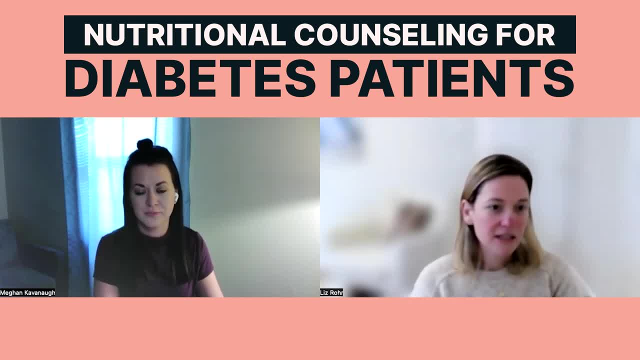 yeah, yeah, because, yeah, because then you add in complications, credentialing, yeah, of like comorbidities with you know ckd. what do you want to think about in those situations? for sure, and i guess the request that you had right was: as long as you don't. 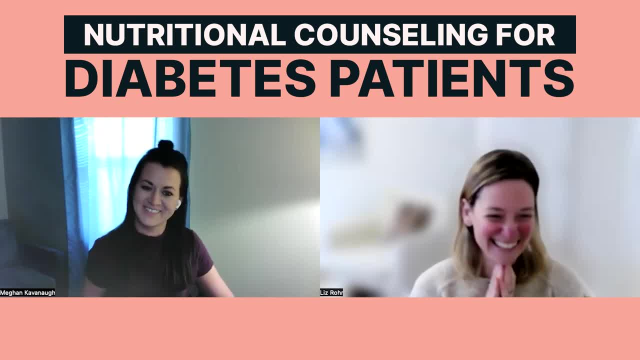 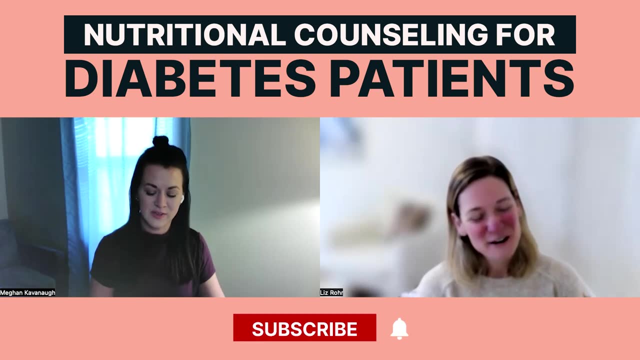 call you a dietary, oh yes, but just don't call me dietary. yeah, so rd works, yes, perfect, yeah, awesome. well, any other parting, uh, words of wisdom, or pearls of practice, or requests, like i said, you know, it's just, i feel, like the overarching answer for like all the questions. 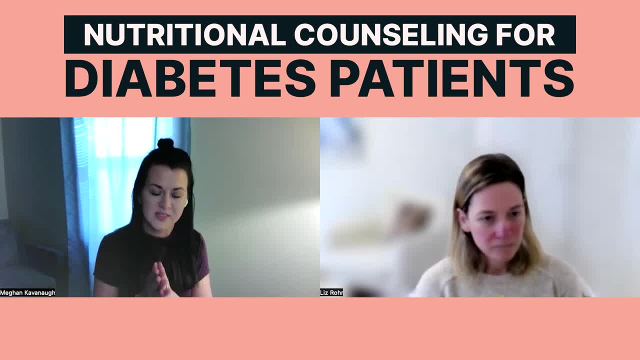 are just that. it depends, and it's just it's okay. if it depends, it's. that's a a hard answer to give because it is just so personalized for every person and it's just. it's just, it's just it's, you know it's. it's just a very unique thing to know and to know that you're not a person that.